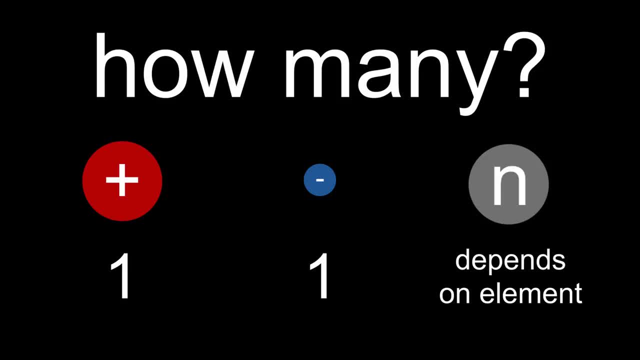 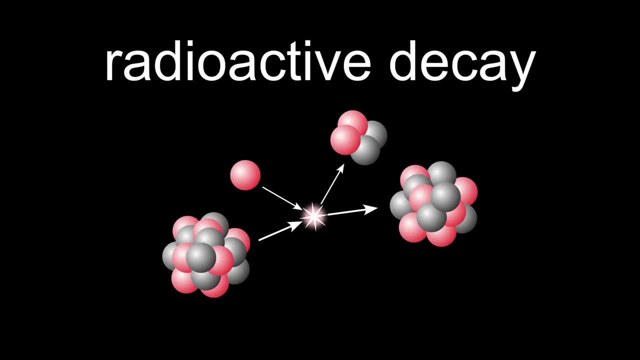 gets bigger from left to right as each element gains a proton, an electron and some neutrons. Depending on the number of neutrons in the core, you get different isotopes of the same element, pretty unstable, and fall apart, releasing ionizing radiation. Fun fact that stuff will kill you. 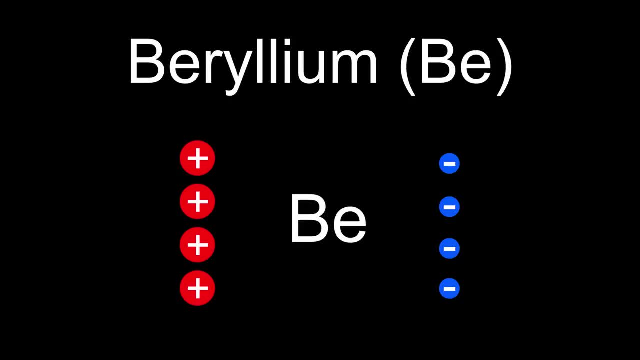 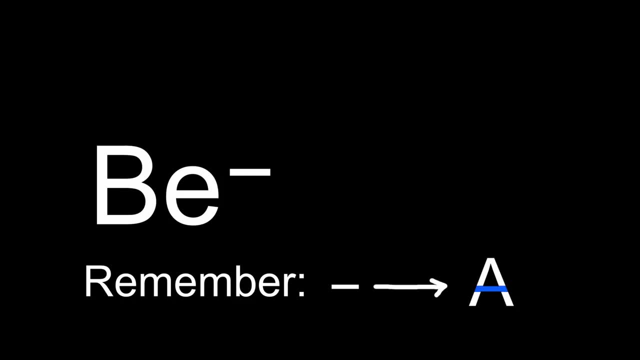 If an atom has the same amount of electrons as protons, it has no charge. If it has more, it has a negative charge and if it has less, it has a positive charge. Charged atoms are called ions, Negative ions are anions and positive ions are cations. 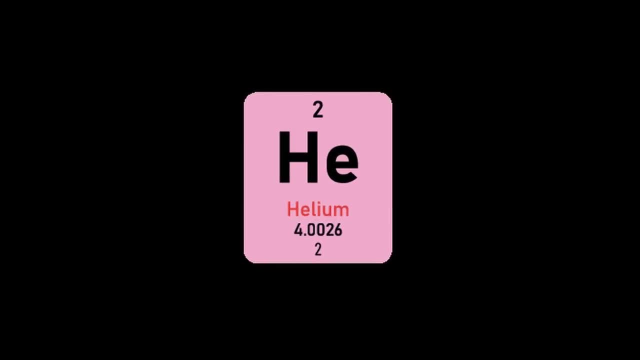 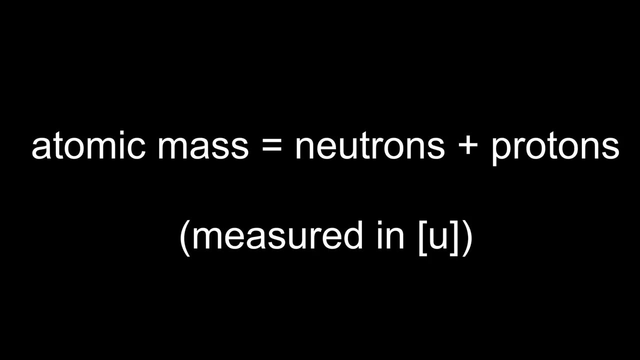 The periodic table is also pretty much a dictionary, as every cell tells you the name and symbol of an element, the number of protons in the core, which is also the total number of electrons, and the atomic mass, which is the mass of neutrons and protons combined. 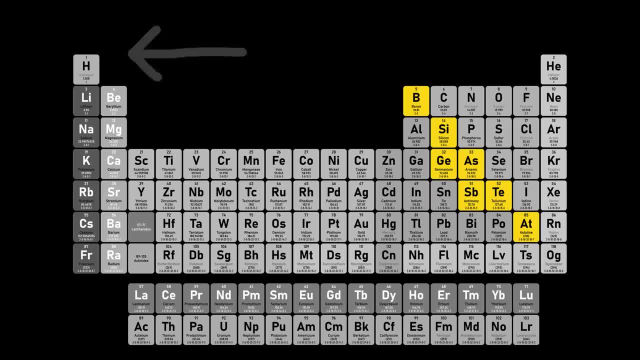 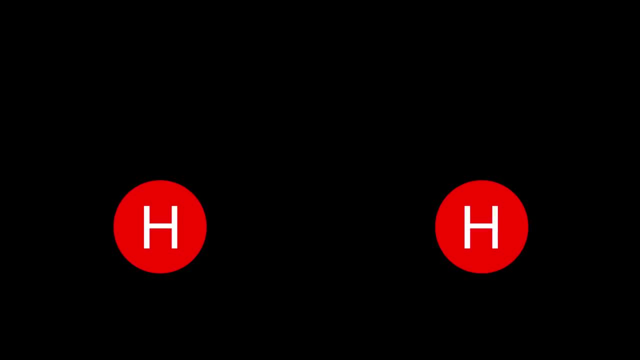 Periodic table is roughly divided into three categories. Left of this line are the metals, right of it are the non-metals, which are mostly gases, and the line is called the semi-metals, which have properties that fall somewhere in between Two or more atoms bonded together. 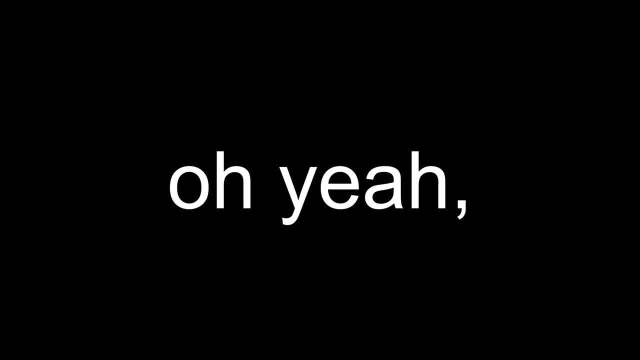 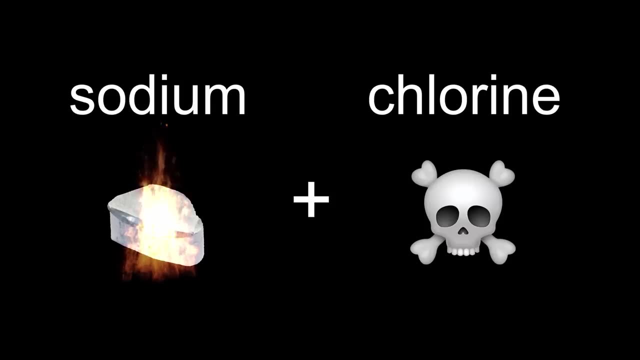 form a molecule. If you have at least two different elements, you get a compound. Oh yeah, this is probably a good time to mention that compounds often behave completely differently than the elements they're made of. Like you put together an explosive metal and a toxic gas. 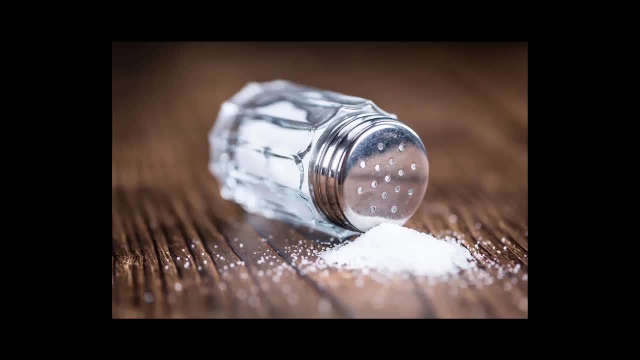 and you get, of course, an even more expl- Table salt. You get table salt. There's many ways to write molecules. For example, if you have an explosive metal and a toxic gas, you get an example of the molecular formula, where you just count the number of each atom in a molecule and 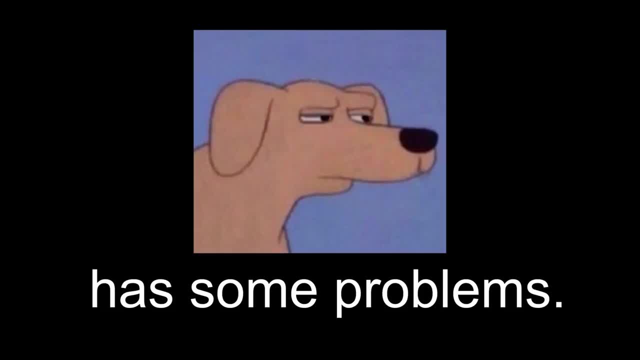 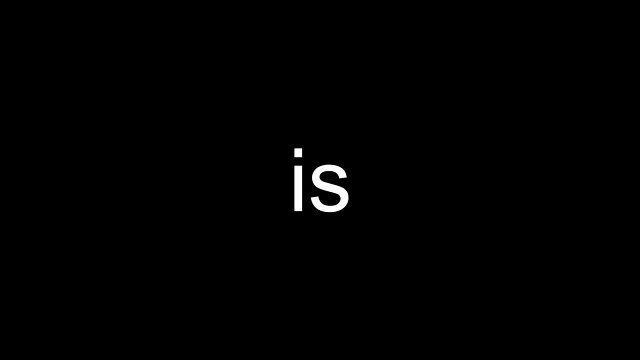 write them as a subscript number next to the element symbol, But that has some problems. Look at these two molecules. They have the same molecular formula, but obviously they're not the same. They're isomers. Showing this difference is probably kind of important. It's the only thing. 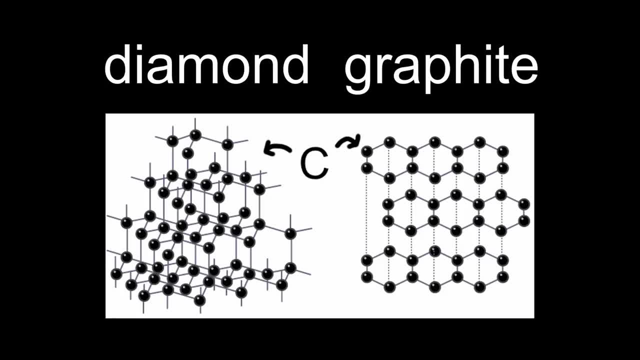 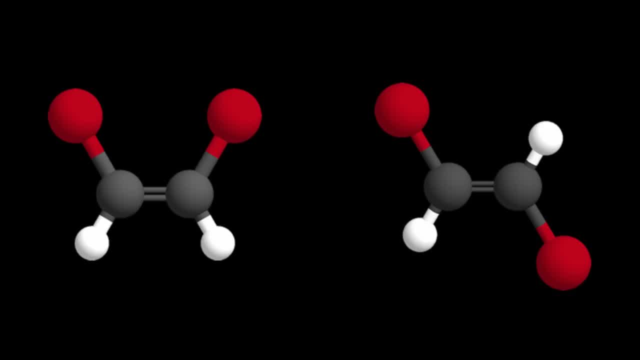 that separates graphite from diamonds, because they're both just fancy versions of carbon and I don't think anyone's gonna go. mmm, yes, this dusty black blob is indeed very expensive. One way to show the structure of an atom is the Lewis dot structure, which represents the valence. 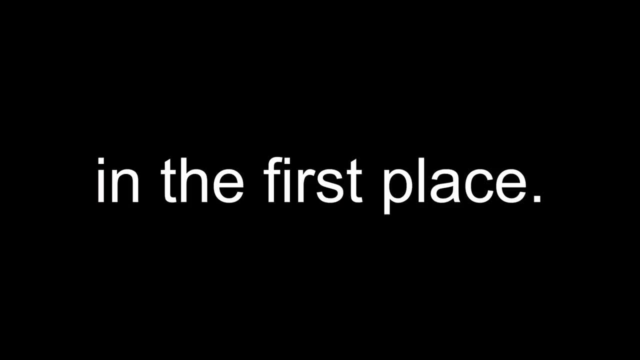 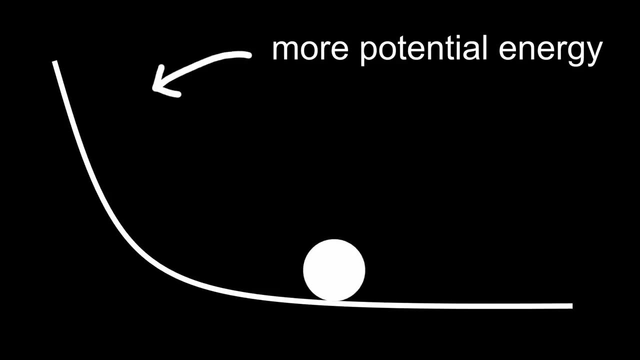 of the atom itself. The valence of the atom itself is the valence of the atom itself. You see, everything in the universe wants to get to a state of lower energy. That's why a ball on a hill will roll down by itself, because that decreases its potential energy. This trend also. 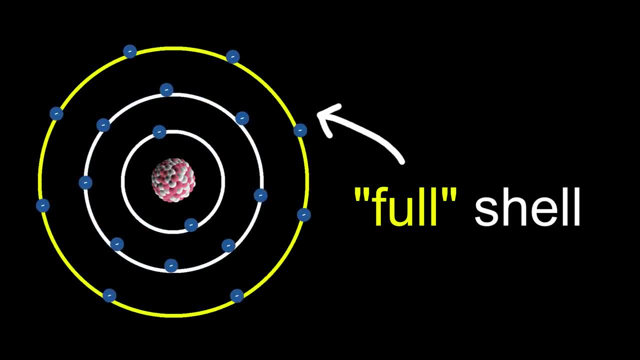 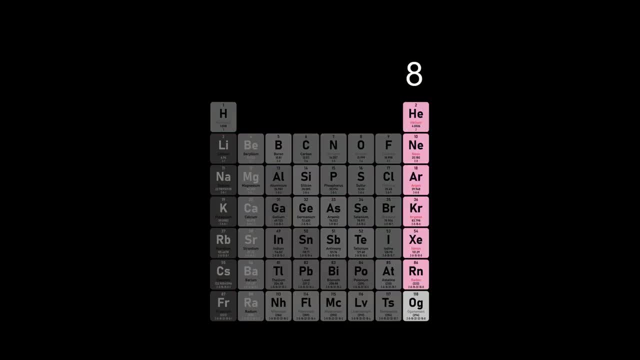 applies to atoms. The state of lowest potential energy is having a full outer shell of electrons, which is most often 8, or, in the case of hydrogen and helium, 2.. If you think back to the periodic table, you'll see that all noble gases already have a full outer shell, which is why they don't. 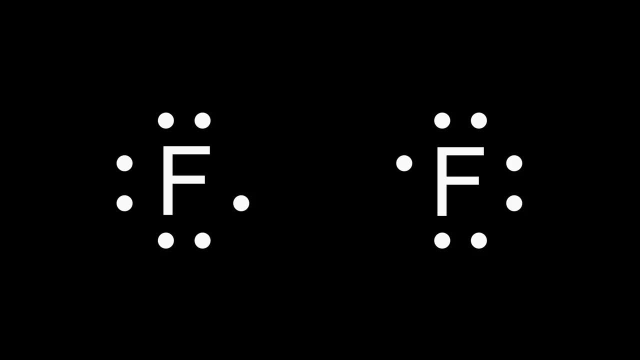 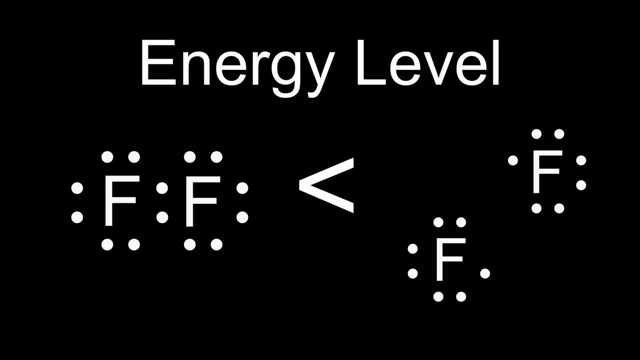 really want to react with anything. If two atoms don't have a full outer shell but can achieve one by sharing electrons, they will naturally do so. the same way a ball will go downhill, as their combined energy would be lower than if they were separate. The sharing of electrons is 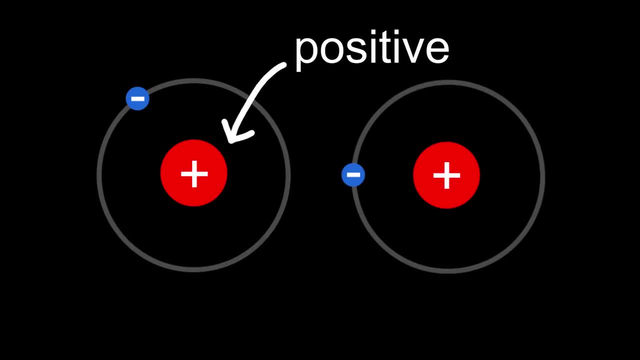 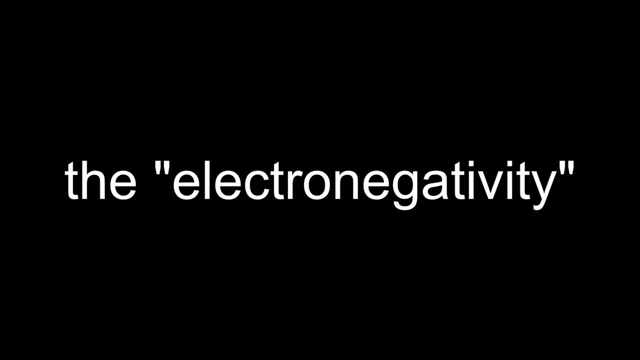 called a covalent bond. These bonds are also caused by the positively charged nucleus of an atom tugging on electrons of another atom. The strength of this pull is called electronegativity. In the periodic table, the electronegativity increases from bottom left to the top right. 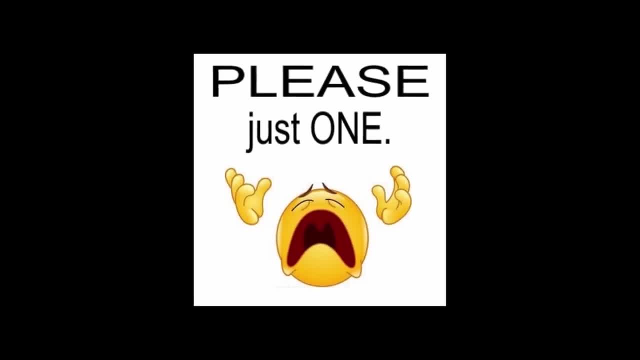 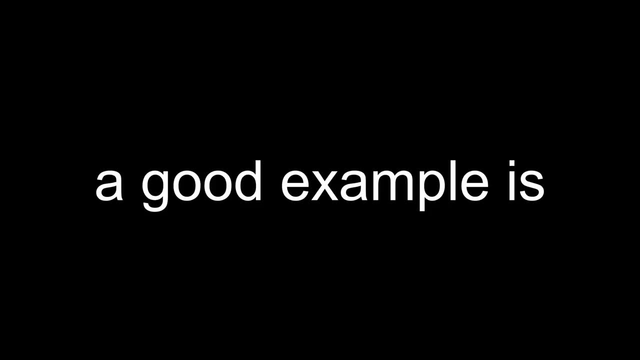 Therefore fluorine has the strongest pull. It's just unbelievably desperate for an electron. If the difference in electronegativity is bigger than about 1.7, you get an ionic bond. A good example is sodium chloride. Chlorine would do anything for an electron. 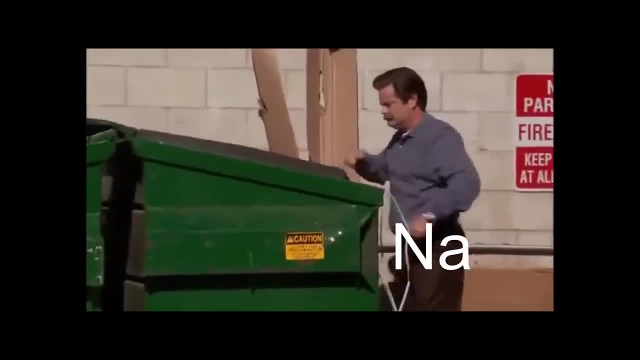 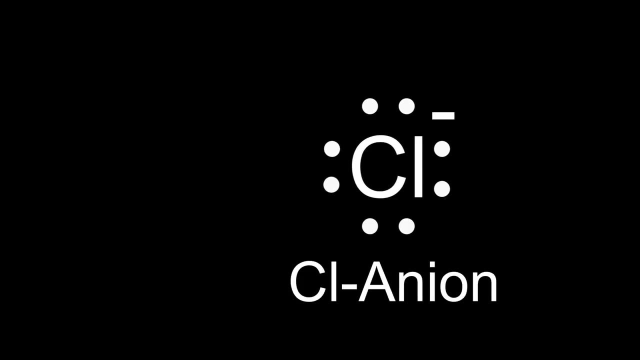 while sodium has one too many and just kinda wants to get rid of it anyway. Perfect, they both say forming an ionic bond where sodium loses an electron and turns into a cation, and chlorine gains an electron and turns into an anion. 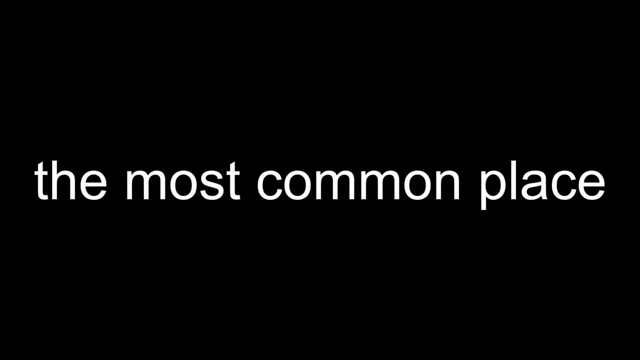 That seems pretty important. You might want to remember it. The most common place you see ionic bonds is in salt. Yes, also table salt, but more generally, when metals and nonmetals bond, you get a salt which is just a grid of ions. 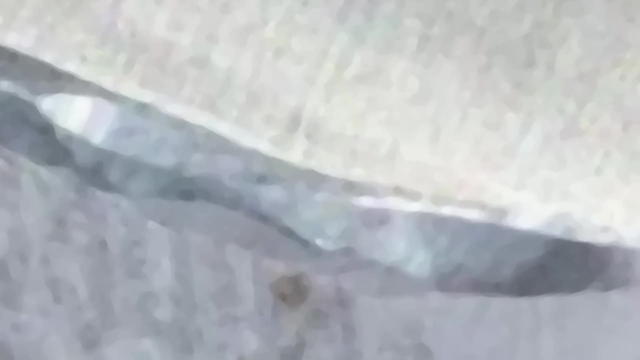 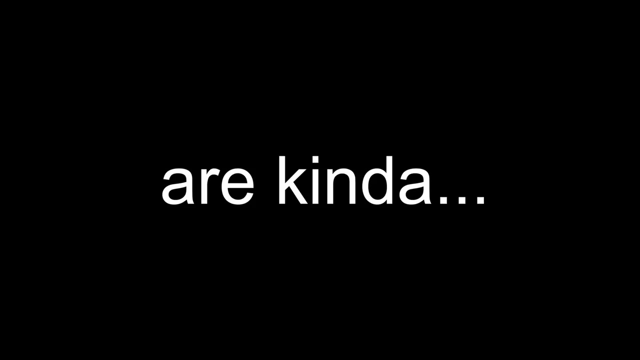 Speaking of metals, a pure metal forms metallic bonds. You can imagine this as a huge grid of positively charged nuclei which are surrounded by freely moving electrons. You see, in a metal grid the valence electrons are kinda promiscuous, or, as the nerds call it, delocalized. They can move freely in a giant playground of nuclei. 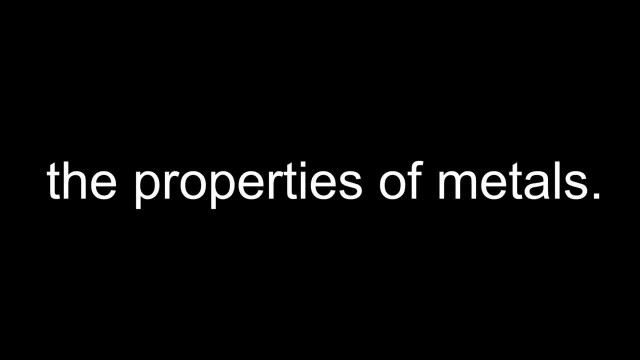 instead of being loyal to just one. This kind of bond is responsible for the properties of metals, like conducting electricity and heat, and also being malleable, as, in being kinda bendy Like you can hammer on this stuff until it's the most deformed. 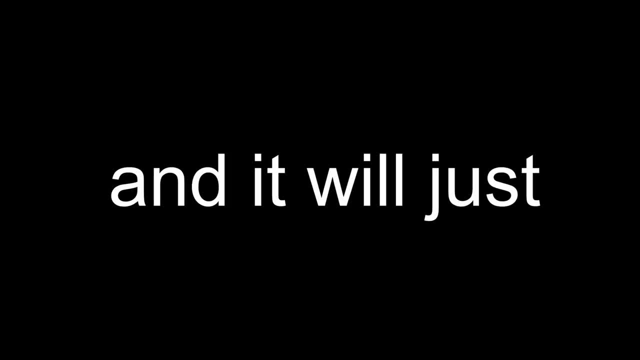 unelegant and ugly looking piece of material ever known and it will just limp along as if nothing ever happened. If the difference in electronegativity is lower than about 0.5, the electrons are shared pretty equally and you get a nonpolar covalent bond. 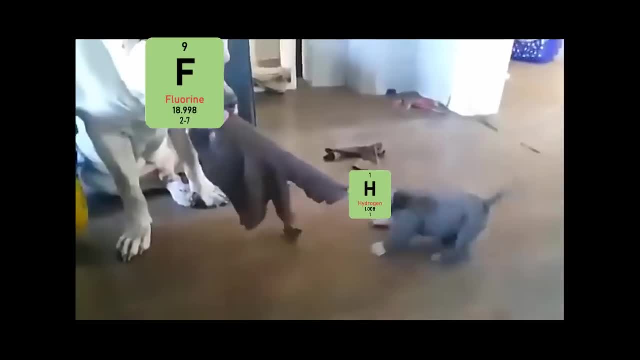 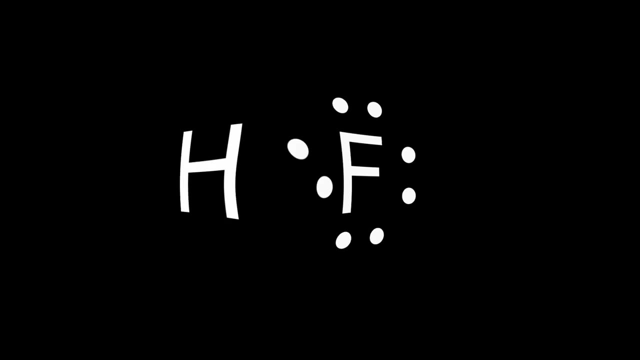 If it's bigger than 0.5, but smaller than around 1.7,. one of the elements is pulling on the electrons pretty hard. Not quite hard enough to completely steal an electron, but definitely hard enough to skew the electrons a bit, making it a polar covalent bond. 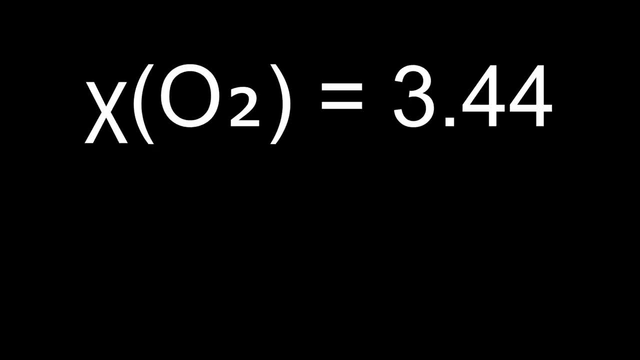 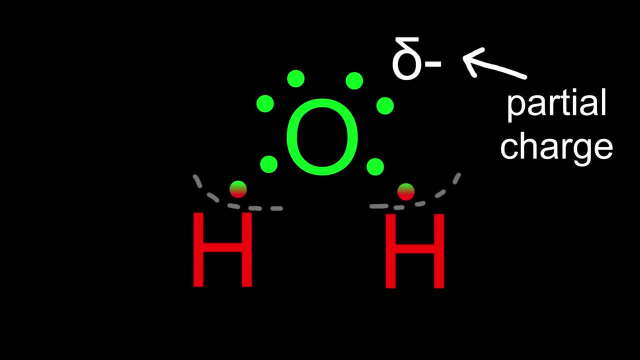 An example is water. Oxygen has a very high electronegativity compared to hydrogen. As a result, it pulls the electrons of hydrogen so hard that they kinda belong to oxygen, giving it a partial negative charge and leaving hydrogen with a partial positive charge. The presence of two poles with opposite charge is called an electric 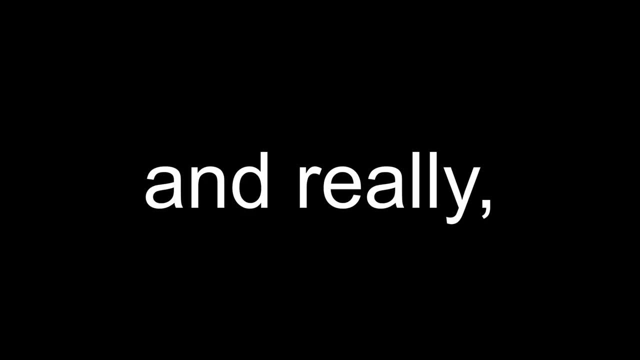 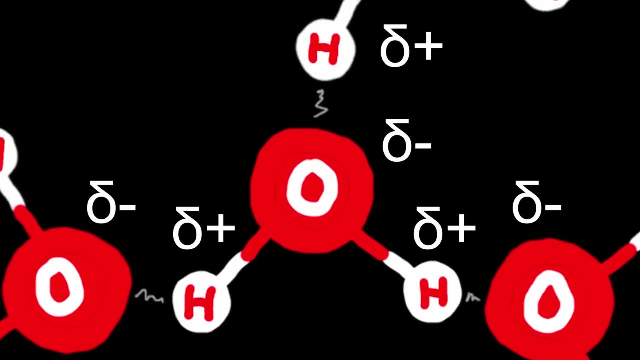 dipole. All permanent dipole molecules can interact with each other and really with anything that has a charge. As a result, the molecules will tug on each other and arrange themselves in a way that oppositely charged ends are next to each other. The forces acting between 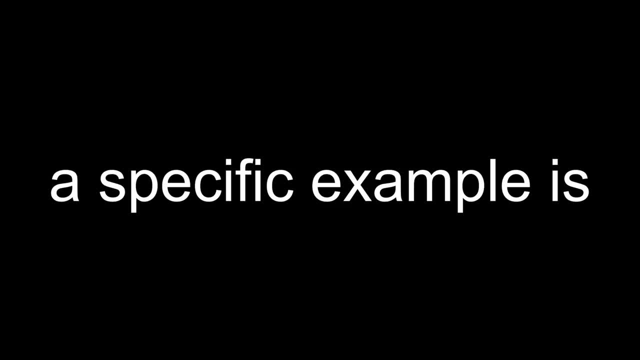 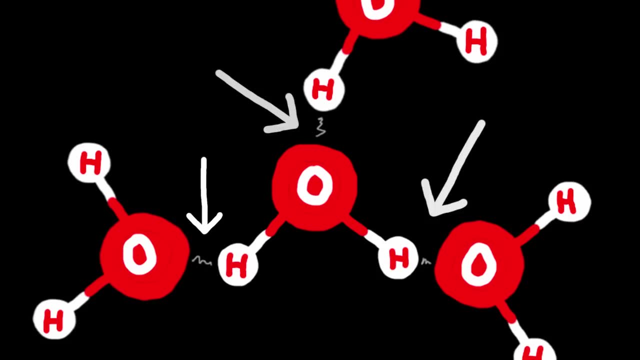 them are called intermolecular forces or IMFs. A specific example is hydrogen bonds, where hydrogen bonds to something very electronegative like fluorine, oxygen or nitrogen, creating strong dipoles that tug on each other. But even if molecules 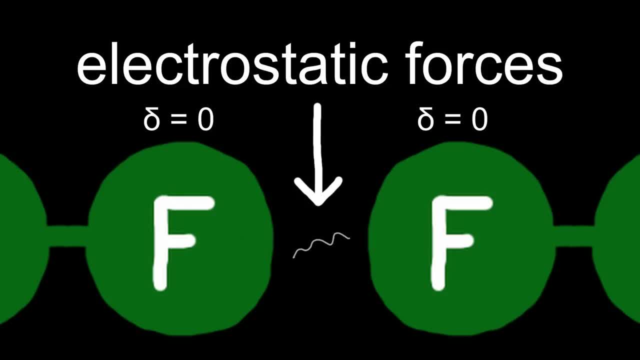 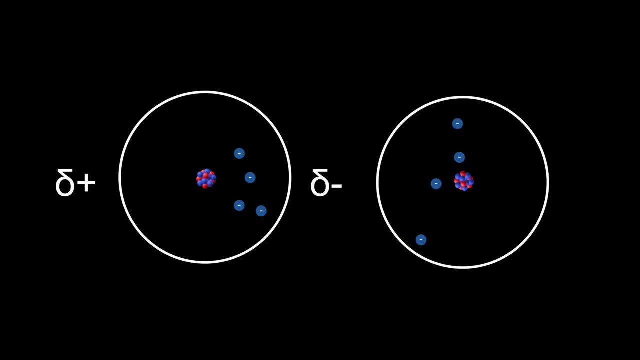 are not polar at all. there can be electrostatic forces acting between them, How Electrons move around inside the atoms and by pure chance they can end up on one side of the atom, creating a momentary dipole which influences other particles next to it to become a dipole. 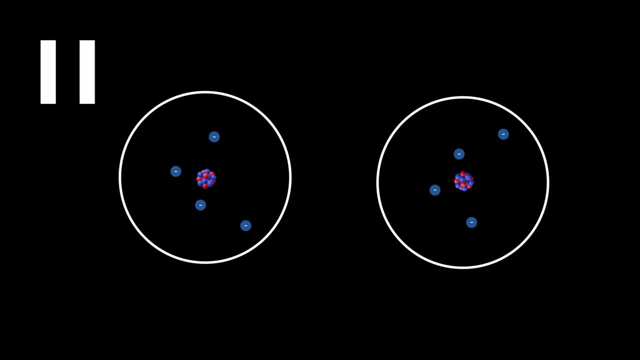 as well, At least for a very short time, as the electrons keep moving and the dipole disappears. This is called the van der Waals forces. The polarity of water also explains why it's one of the most versatile sources of energy in the universe. The polarity of water also explains why 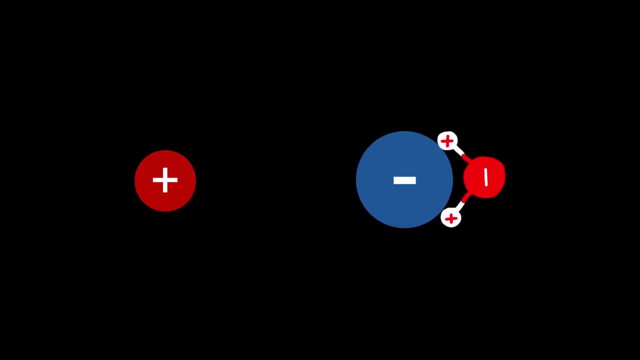 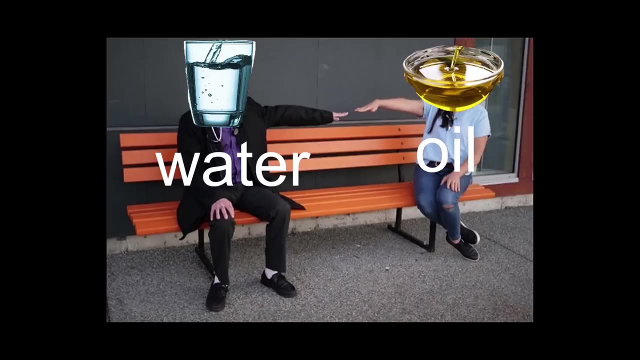 solvents exist. It can pull apart molecules by tugging on charges, and it keeps them apart by surrounding a particle with its oppositely charged end. Water cannot dissolve non-polar molecules, though. It's the reason why water and oil don't mix. 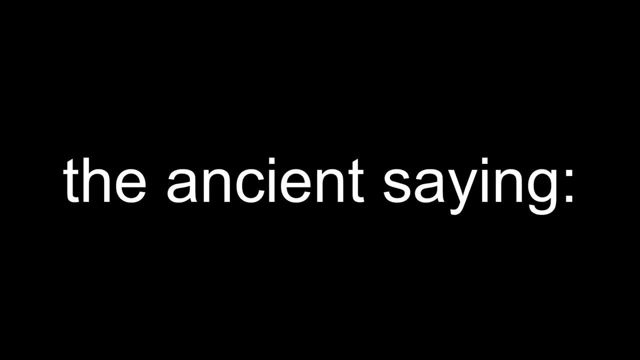 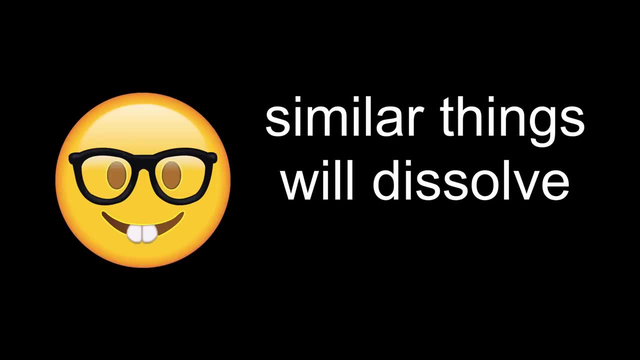 since fat molecules are non-polar, while water is polar. Just remember the ancient saying similia similibus solventum, or in the language that's actually spoken: similar things will dissolve similar things. Fun fact: Soap works because the molecules that 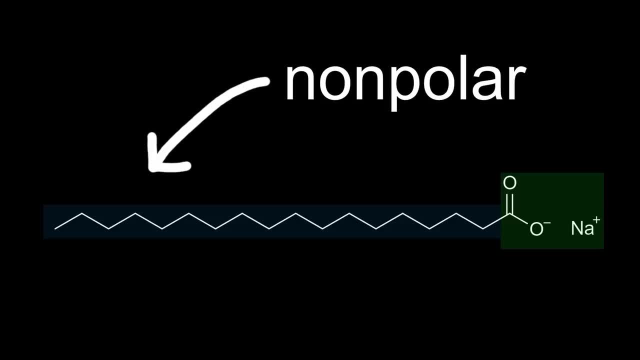 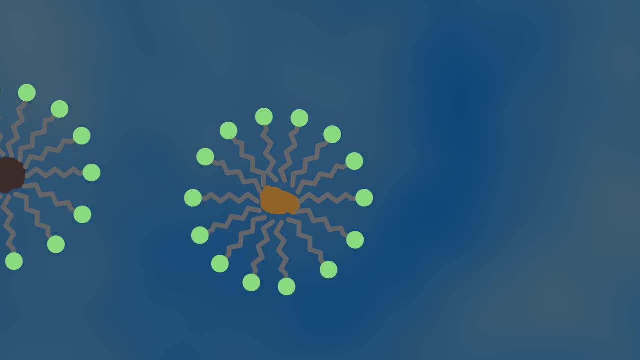 it's made from, which are called surfactants, have a polar head and a non-polar tail. This way, when in water, they can surround, for example, non-polar fat molecules and form micelles which, along with the water, transport the dirt particles away. 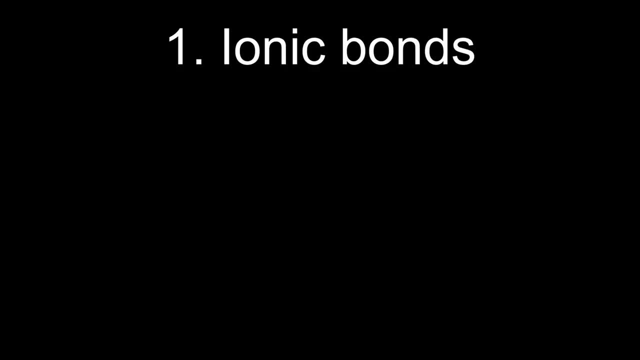 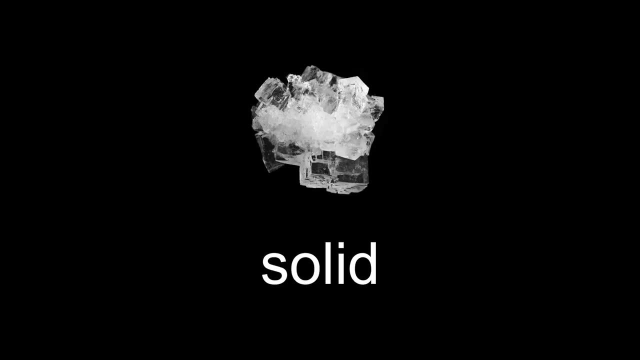 These are the most important bonds and forces, ranked by strength: Ionic bonds, covalent bonds, metallic bonds, hydrogen bonds and van der Waals forces. There are three main states of matter: solid, liquid and gas. Solids are tightly packed in fixed structures. 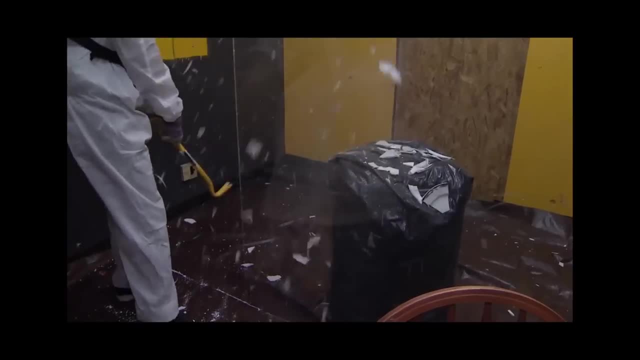 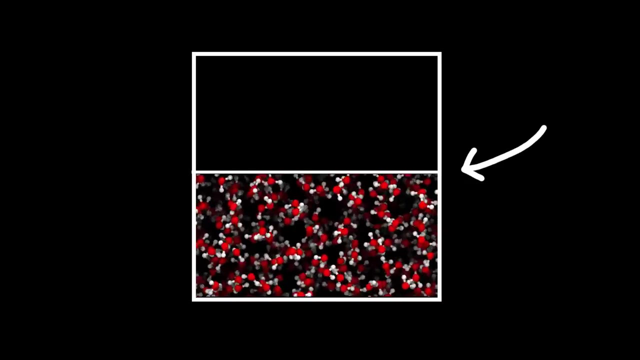 where the particles can only wiggle, Unless you know you smash them. In liquids the particles can move freely, but are still confined to a fixed volume, as the forces between them are still strong enough to keep them together And the particles in gases have enough energy to just do whatever they want. 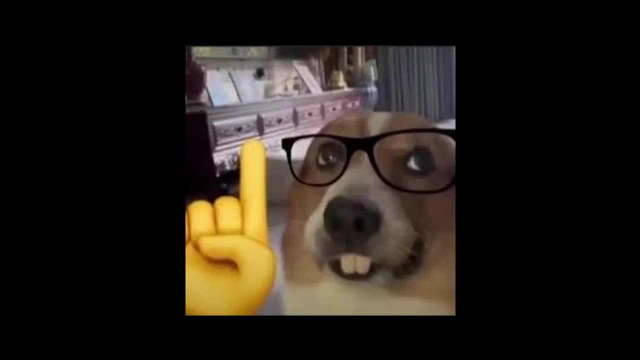 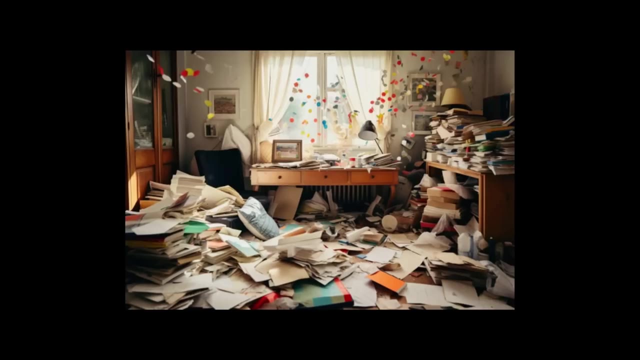 and fill up all the volume you give them. Knowing this, we can find two important words: Temperature is the average kinetic energy of particles in a system, or how much and how fast they move, and entropy is the amount of disorder. Substances tend to be solid at low temperature and or high pressure. 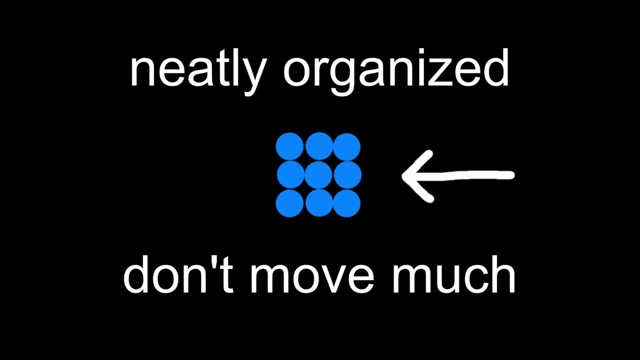 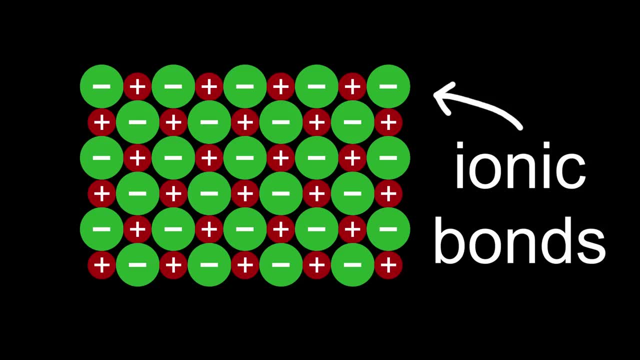 which is a state of low entropy, as they're neatly organized and don't move that much, and gas at high temperature and or low pressure where they move around like crazy, so it's a state of high entropy. Strong bonds, like ionic bonds, lead to high melting points as they take a lot of. 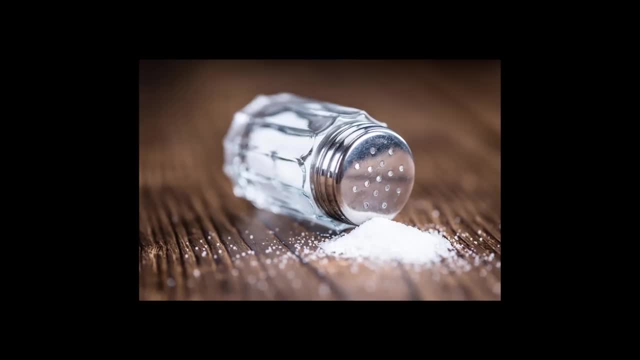 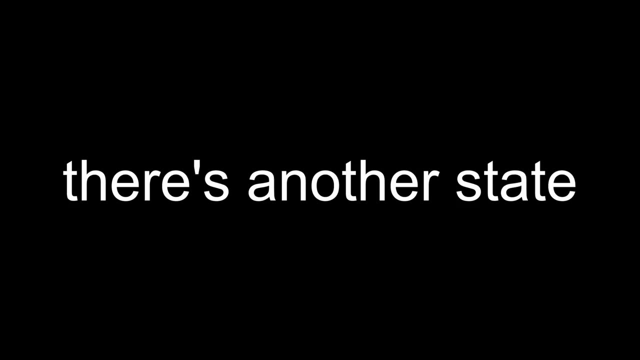 energy and therefore a high temperature to break apart. That's why most salts are solid at room temperature, whereas water, which is only being held together by hydrogen bonds, is a liquid. Well, actually, there's another state, called plasma, which is ionized gas and can exist. 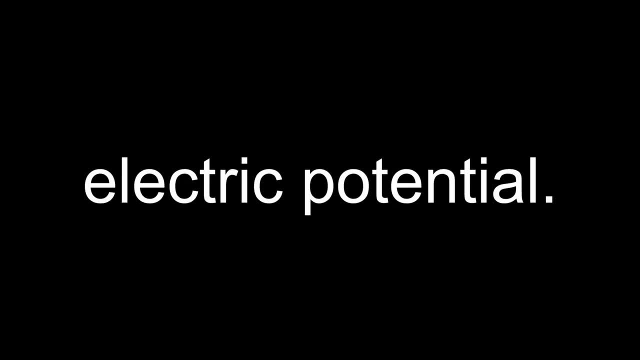 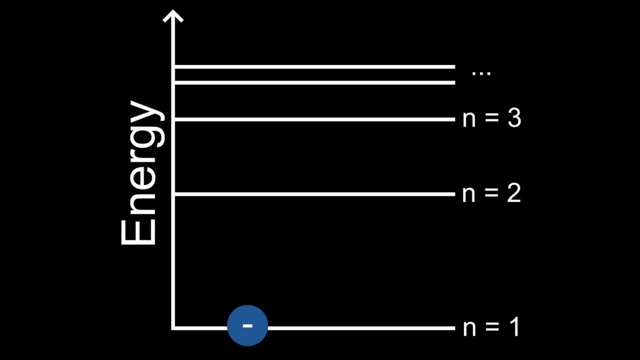 at very high temperatures, such as in stars, or very high electric potential. The latter is used for neon lights. Gas is ionized in a tube with a very high voltage. Collisions of the ions with other particles makes their electrons move to a higher energy state. 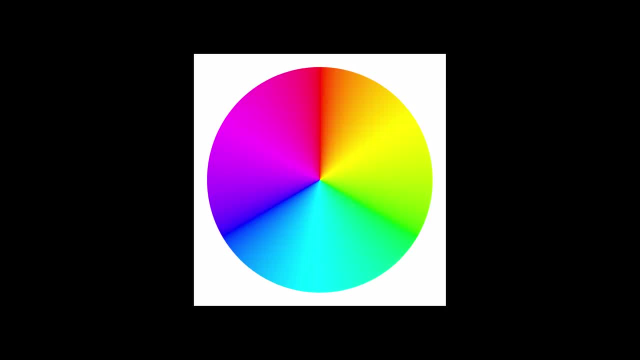 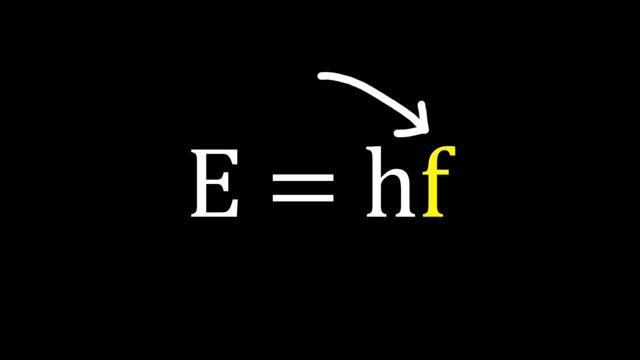 Once they fall back down, the difference in energy is released as light. The color of the light changes depending on the element that's used in the tube, as each element has different but fixed energy levels, and the difference between those determines the energy and therefore the frequency. 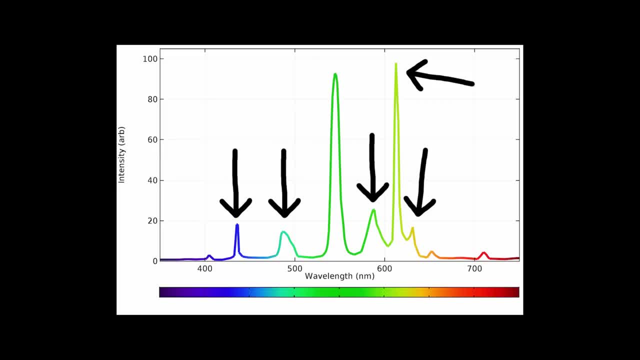 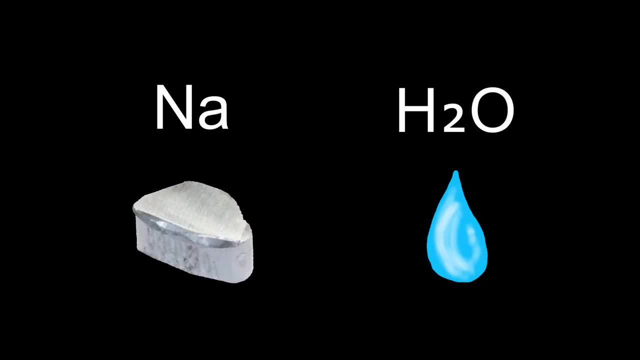 of the released light, which is what changes the color. All possible frequencies that an element can emit are called the emission spectrum. All matter can be divided into two categories: pure substances, which can consist of one element or one compound, and mixtures. Mixtures consist of: 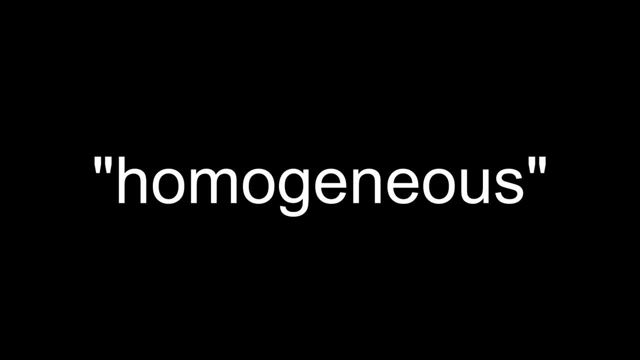 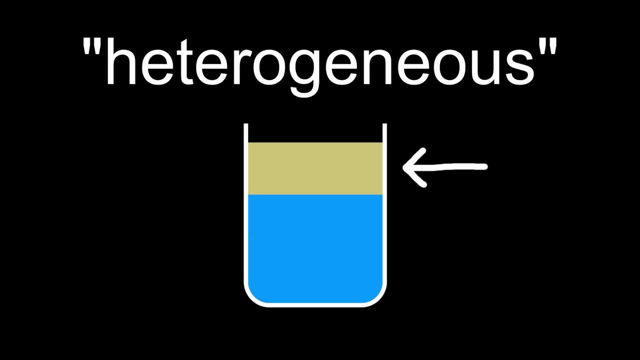 at least two pure substances and can be homogeneous or heterogeneous. Homogeneous means the substances will mix evenly and the mixture looks the same everywhere, like salt and water, which is a heterogeneous mixture. Heterogeneous mixtures look different depending on where you look They. 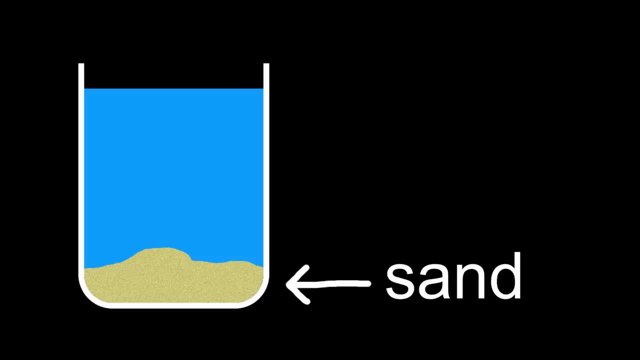 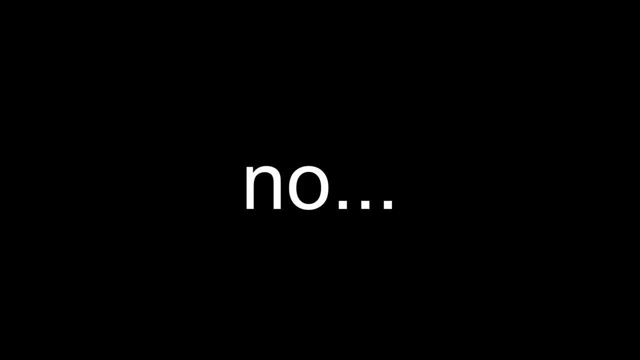 have distinct regions made of separate substances. One example is sand and water, which is called a suspension. Okay. well, what about milk? That looks the same everywhere, so it must be homogeneous. Uh, no, Milk is something we call a colloid, or, more precisely, an emulsion. The difference? 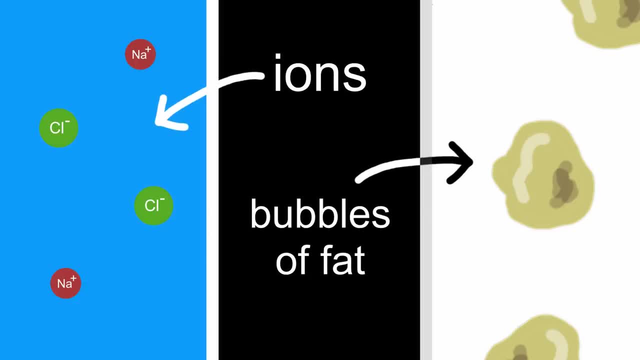 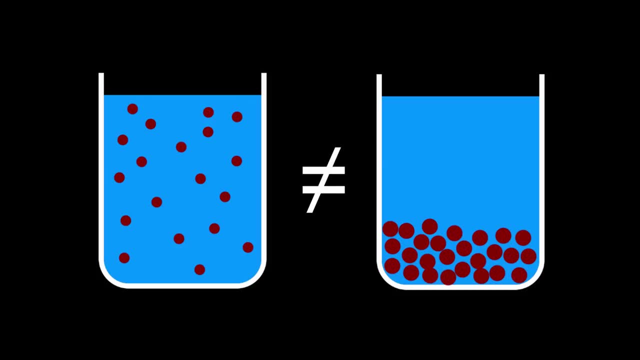 between salt water and milk is that the solute doesn't fully dissolve in the solvent, meaning there are bigger particles than in a solution but smaller particles than in a suspension. This allows the particles to stay evenly distributed but not fully dissolved, placing them somewhere. 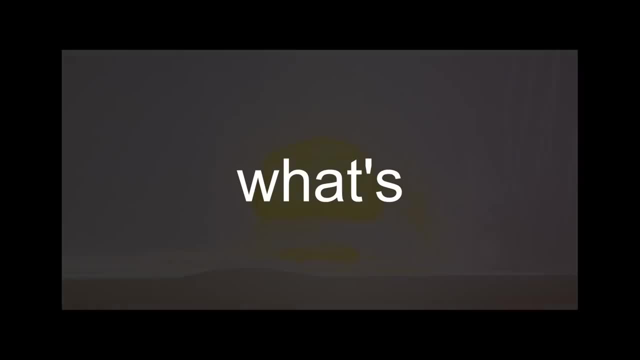 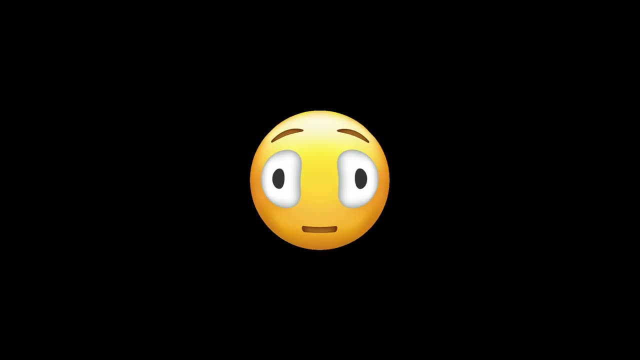 between solutions and suspensions. Hey, remember sodium and water. What's going on there? Explosions are really just chemical reactions that release a lot of energy in a very short amount of time. Also, they expand Like a lot. There's a couple types of chemical reactions. 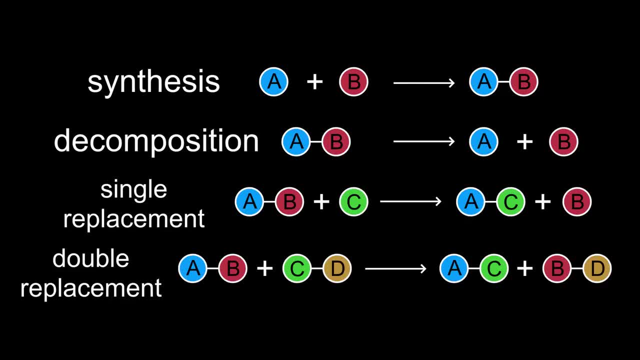 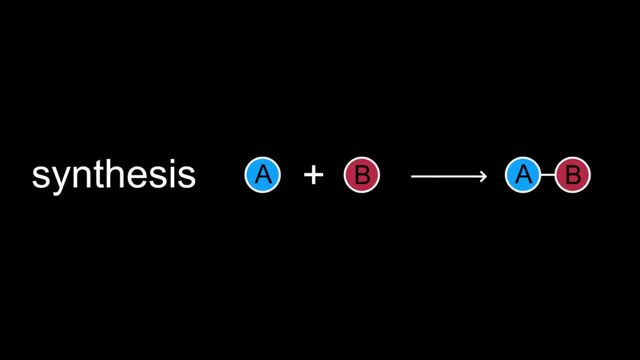 Synthesis, decomposition, signal replacement and double replacement. Here's an example for each one. They all happen mainly for one reason: to decrease energy and get to a more stable state. Chemical reactions happen in certain ratios, For example to produce water molecules. 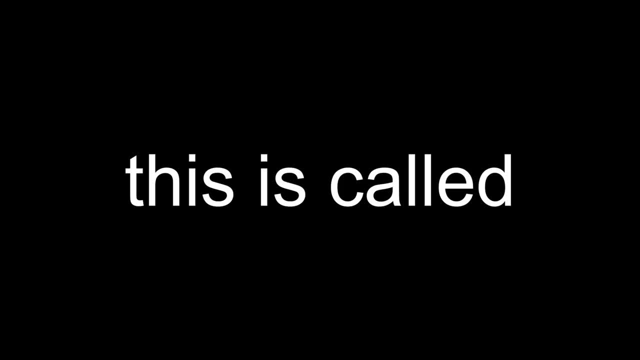 you need twice the amount of hydrogen compared to oxygen. This is called stoichiometry. These ratios are based on the conservation of mass, which says that mass cannot be created or destroyed, only converted. Practically, when dealing with reaction equations, you have to make sure that there's the same amount of 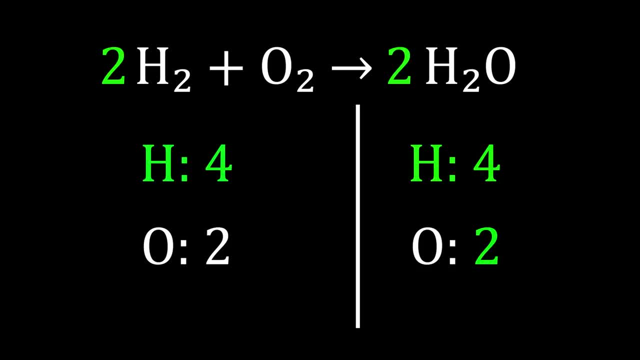 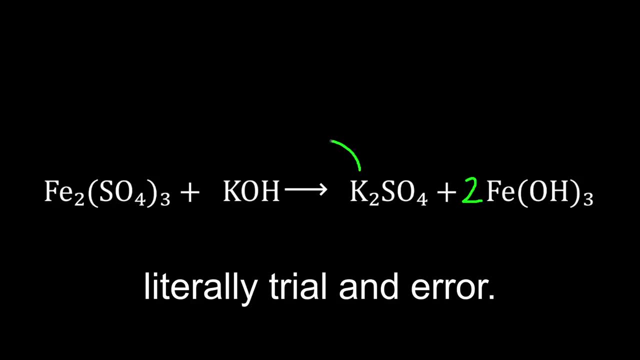 atoms on each side of the equation and, if not, balance it out element by element. As a rule of thumb, you should balance out the metals first, then the non-metals and then hydrogen and oxygen at the end. But it's really just trial and error until everything is balanced. Okay, but if you 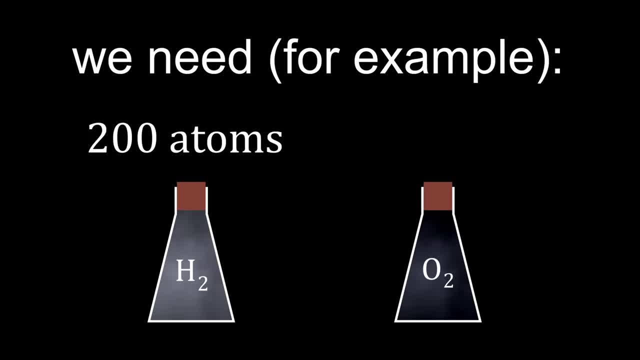 wanted to make this reaction happen in a lab, how would we know that we have exactly twice the amount of hydrogen compared to oxygen? Well, that's a good question, but it's not a good question. You can't just take 10 grams of this and mix it with 20 grams of that, because the atoms don't. 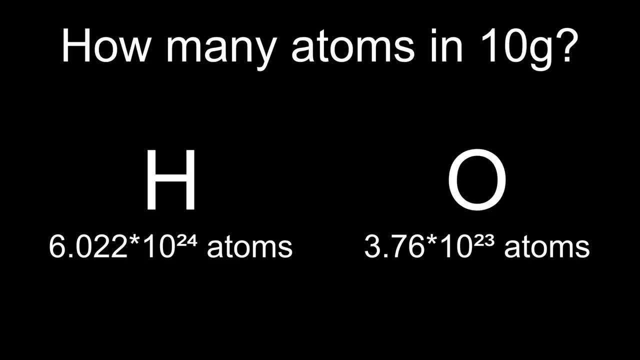 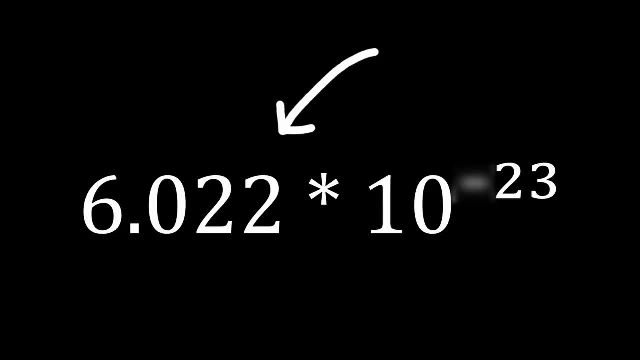 weigh the same, so 10 grams of both contain a different amount of particles. What to do? Just look up the atomic mass of the reactants and take that amount in grams. You'll get exactly this amount of particles. That is one mole which is just an amount of something kind of like a. 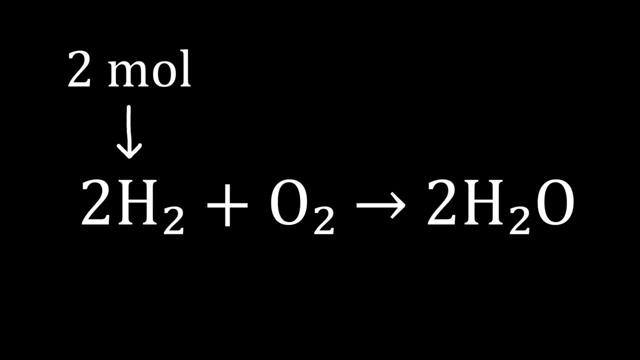 dozen. In other words, we can interpret the reaction as two moles of this react with one mole of that which we can easily measure. It's important to differentiate between physical and chemical changes, as reactions only take place in the latter, Physical. 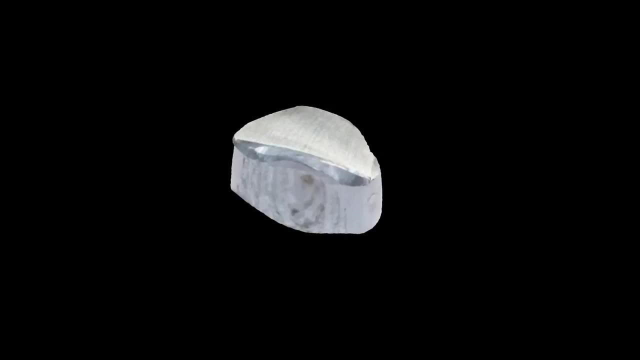 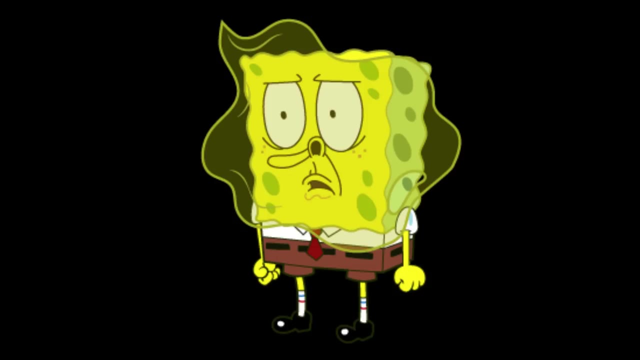 change happens when the appearance changes but the substance does not, For example, hammering metal. A chemical change happens when the substances themselves change, and this is often accompanied by bubbles, a funky smell or- you guessed it- explosions. All chemical reactions. 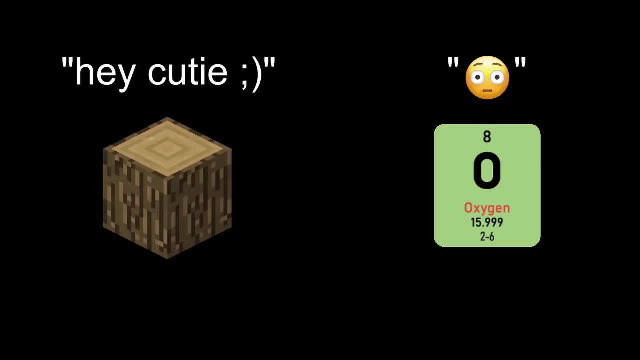 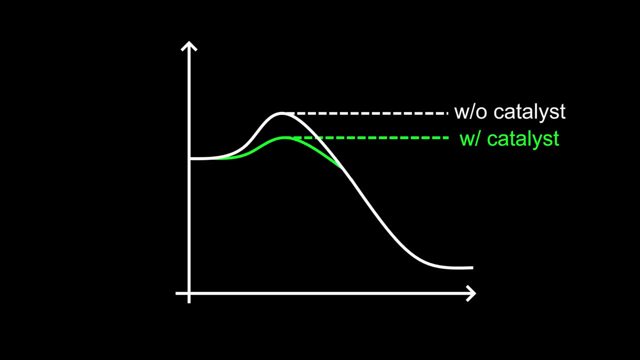 need activation energy to take place. Wood won't just spontaneously react with oxygen and start burning, or else, you know, the planet would be on fire. but if you give it enough energy, it will, Catalysts, reduce the activation energy needed for a reaction which makes it happen. 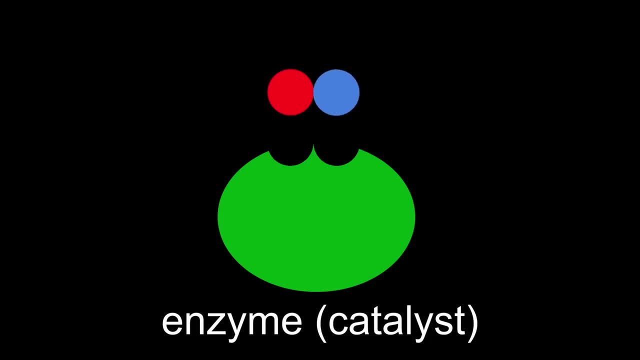 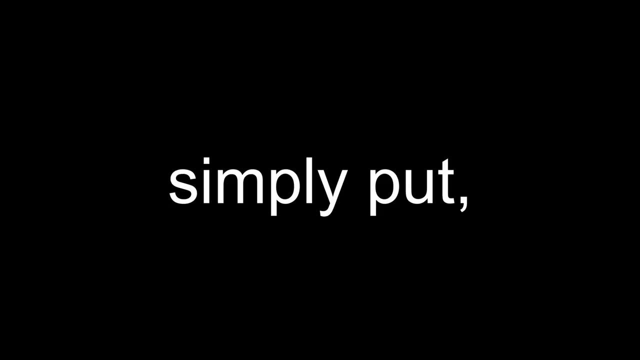 easier and faster And as a neat bonus, they don't even get used up during the reaction, so you can just reuse them. Because chemical reactions are changes in energy, it's quite useful to keep track of it. Enthalpy is, simply put, the internal energy or heat content of a system. If the total 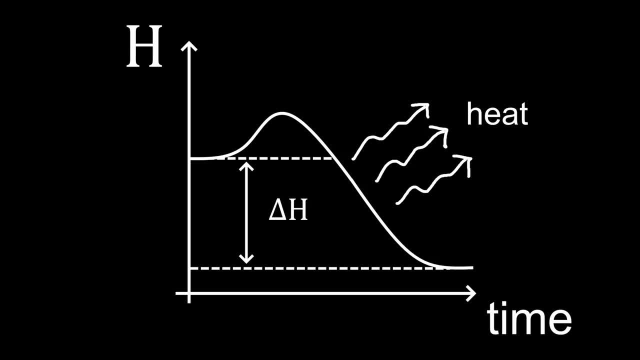 enthalpy of a reaction is lower at the end than at the beginning. heat was given off to the surroundings, which is an exothermic reaction. If it's the other way around, a reaction is endothermic. It's easy to see how exothermic reactions can be spontaneous. It's kind of like a 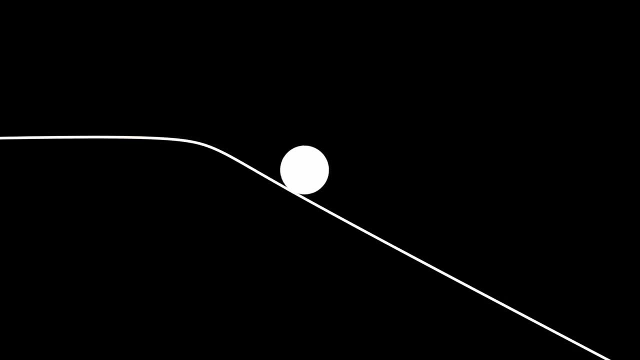 ball on a hill, It will only start rolling if you push it a little bit, then it will keep rolling on its own, just like wood keeps burning on its own, But in endothermic reactions you have to keep putting in energy, like pushing a ball uphill. 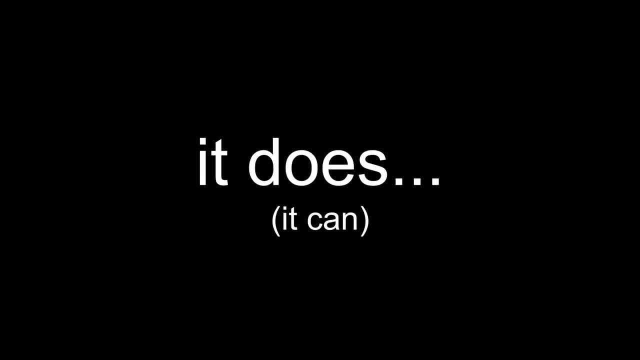 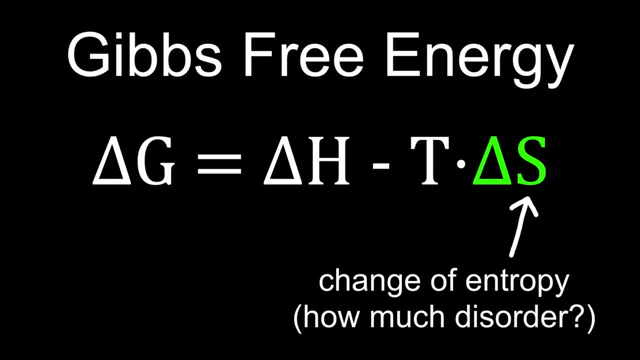 That doesn't just spontaneously happen, right? Well, yes, actually it does. To get the whole picture, we have to look at Gibbs free energy, which looks at the change of enthalpy, but also the entropy of a system which is dependent on temperature, If this whole thing is less than zero. 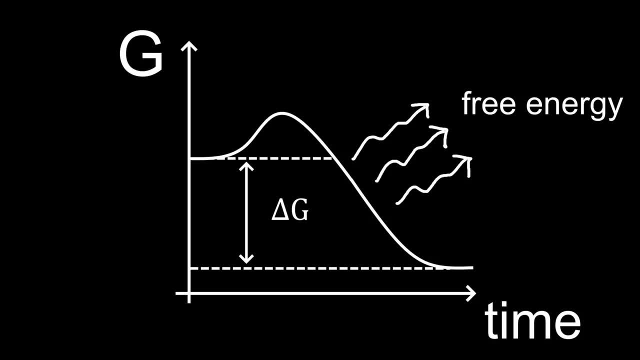 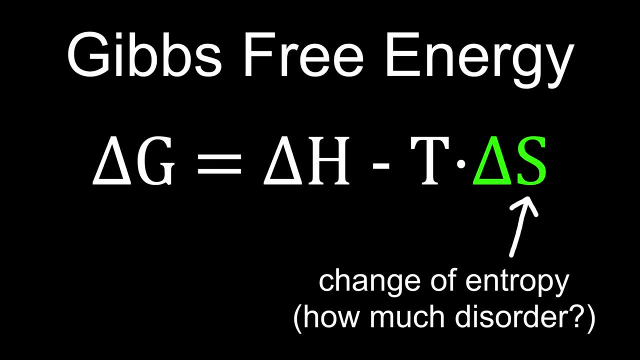 the reaction is exergonic or spontaneous because free energy was released. If it's bigger than zero, it's endergonic or not spontaneous because free energy was needed and absorbed. Here's where temperature and entropy come into play, Even if delta H is positive. 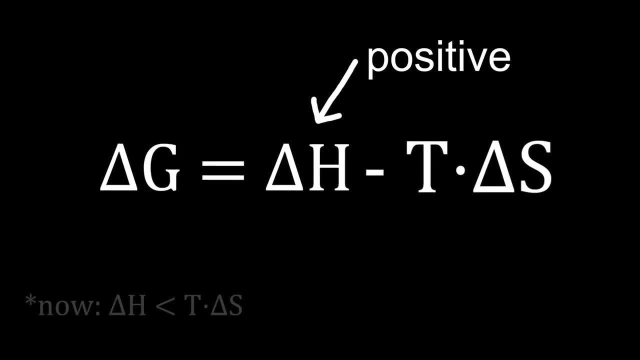 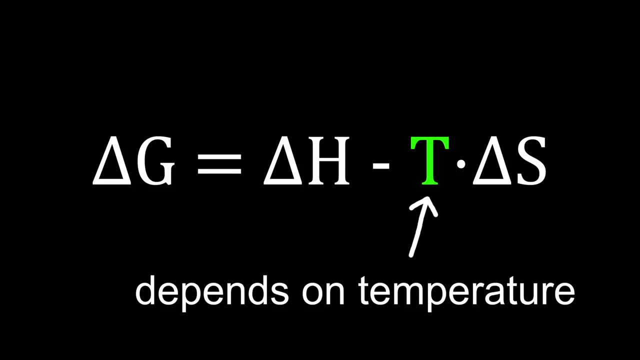 so the reaction is endothermic. if the change in entropy is big enough, it can offset this and make the total free energy negative, which means the reaction is spontaneous. But this is strongly dependent on the temperature. For example, melting an ice cube is endothermic because it absorbs. 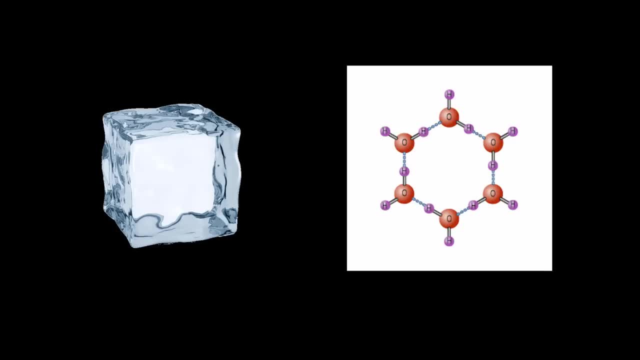 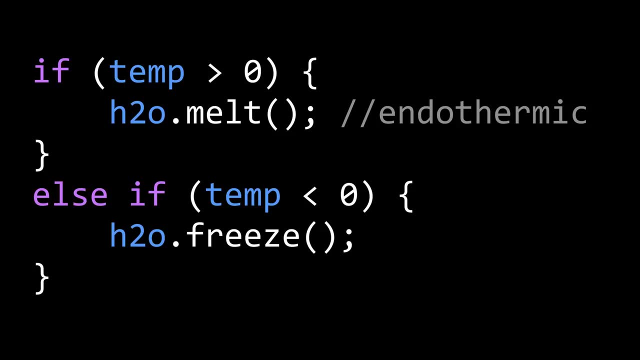 heat, But also it increases the entropy a lot, as neatly organized ice turns into water, which is just kind of a mess. So this can happen spontaneously, but only if the temperature is above zero. If it's below zero, the water will spontaneously melt. 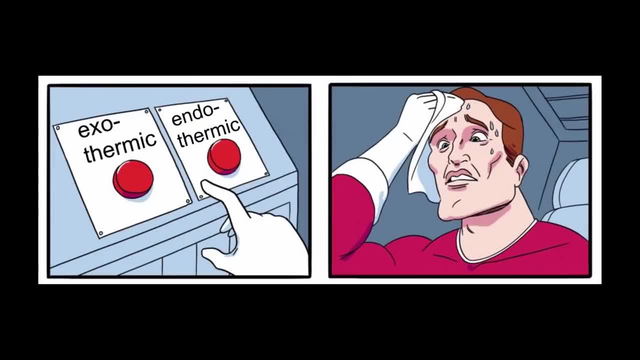 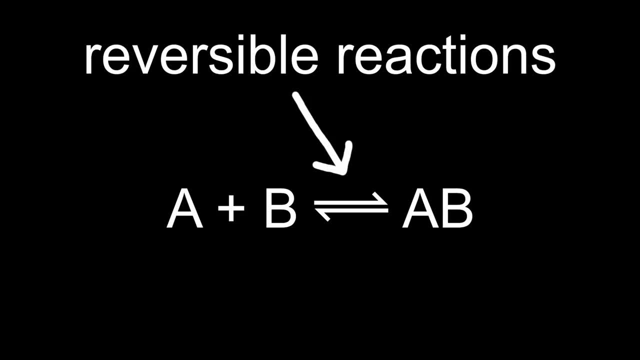 If it's exactly zero, then no reaction will take place spontaneously. In other words, if delta G is zero, we're at equilibrium. Chemical equilibriums exist when reversible reactions take place at the same speed in both directions, which means that even if reactions 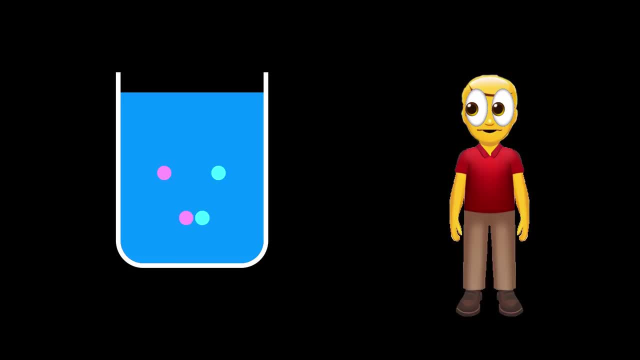 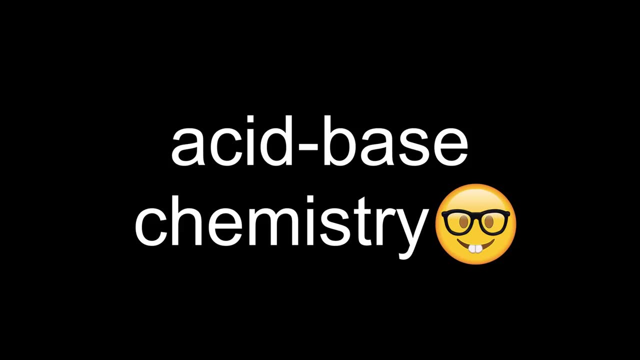 are taking place. the concentrations of both sides stay the same and to someone watching from the outside, nothing seems to be happening. We often find chemical equilibriums in phase changes, but also acid-base chemistry. According to Brensted-Lowry, an acid is a molecule that 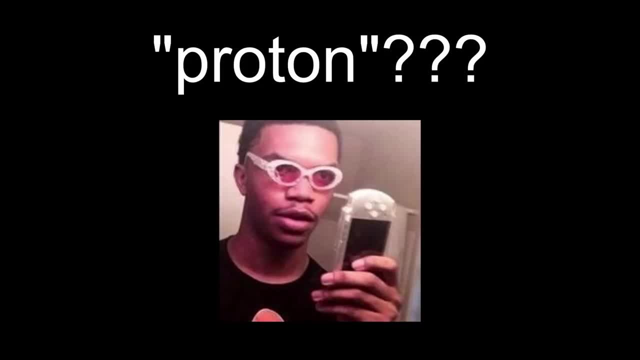 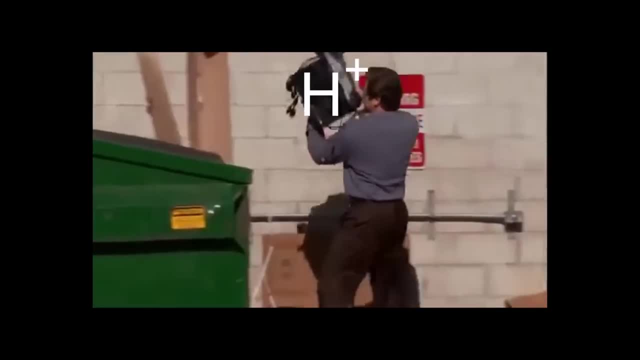 donates protons, while bases accept protons. A proton in this case is just a hydrogen ion. So with this definition, a molecule with at least one hydrogen that it can throw away can be an acid and anything that can pick it up can be a base. This also means that once they react, 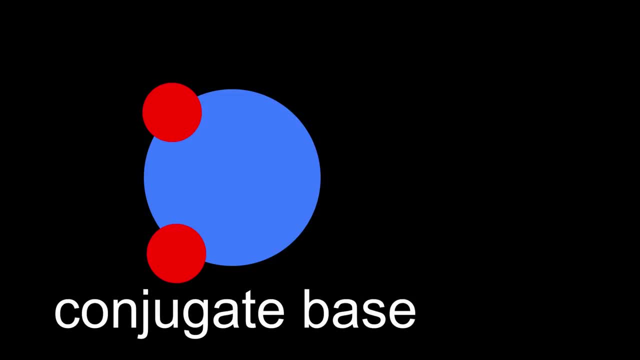 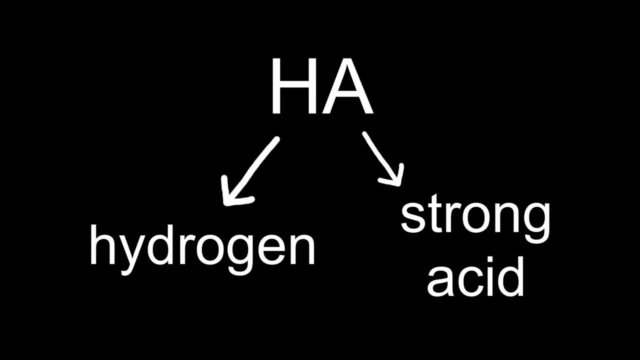 they turn into the conjugate opposite, as an acid that gave away a proton can now accept one back, which is what bases do. A molecule that can act as both an acid and a base is amphoteric, for example, water. A strong acid will dissociate almost completely into its ionic form, giving off a lot of protons to the water and therefore create the reaction of a solid as an ionic form. The reaction of a solid is called the reaction of a solid and the reaction of a based ionic form is called the reaction of a solid. The reaction of a solid is called the reaction of a solid and the reaction 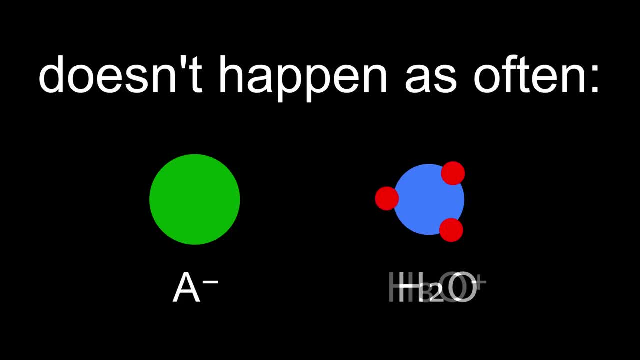 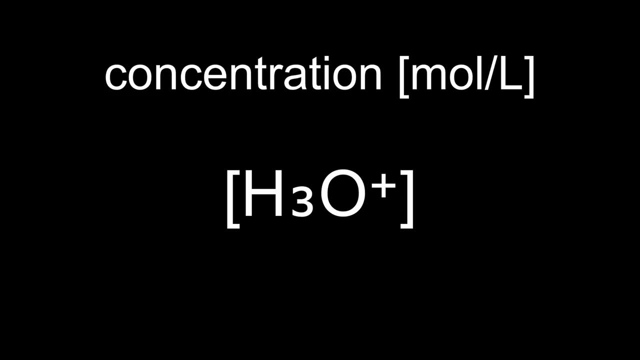 we're creating lots of hydronium ions. A weak acid just won't dissociate nearly as much, giving us a lower concentration of hydronium ions. So to measure the strength of an acid, we can measure the concentration of hydronium ions. This is called the pH. Mathematically it's defined as: 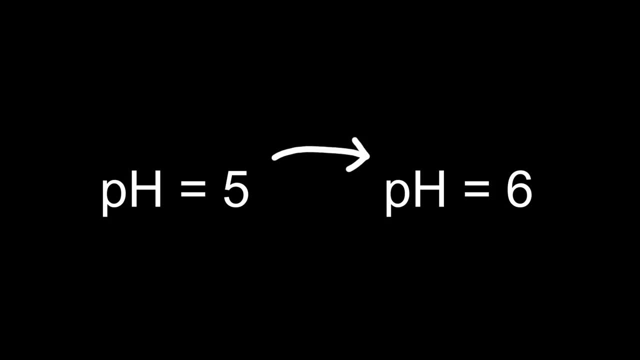 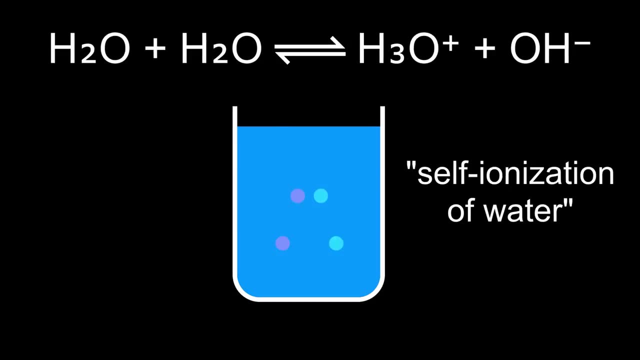 the negative log of the hydronium concentration, which means one step on the scale, is a 10 times change. And also, since it's a negative log, the higher the concentration, the lower the pH. For example, pure water is. in a chemical equilibrium There's exactly one hydronium. 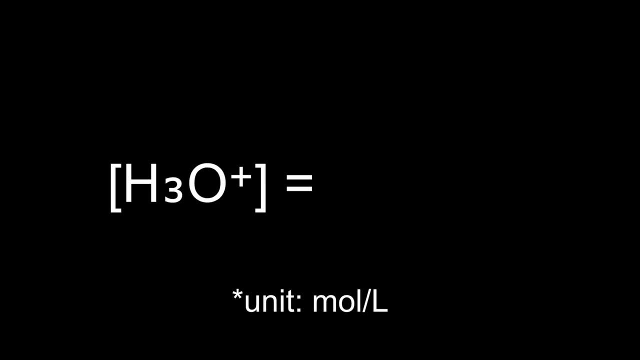 ion for every 10 million water molecules. In other words, the concentration of hydronium is 1 over 10 million, or 1 times 10 to the negative 7.. Taking the negative log of this gives us a pH of 7, which is considered neutral. Anything lower than 7 is acidic. 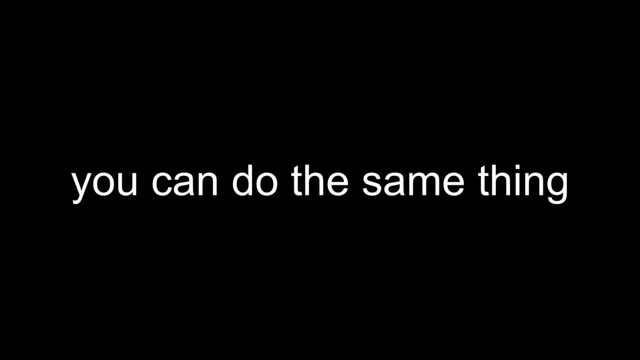 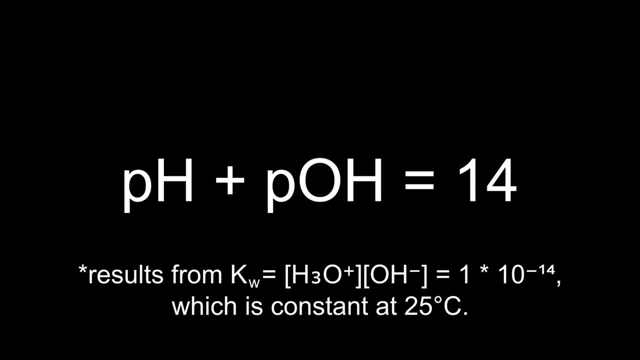 and anything above is basic. unlike you, You can do the same thing with hydroxide ions and you will get the pOH, which keeps track of basicity. Fun fact, the pH and pOH will always add up to 14, because they counteract each other. So by knowing one, you know both. 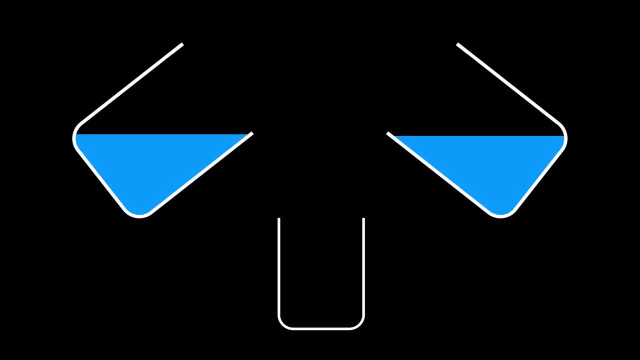 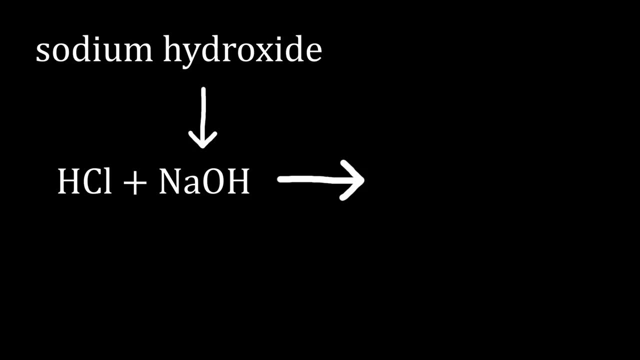 Now, if you have a strong base and a strong acid and you pour them together, no, they will not explode. They will neutralize by forming water along with the salt which is neutral, For example hydrochloride and sodium. 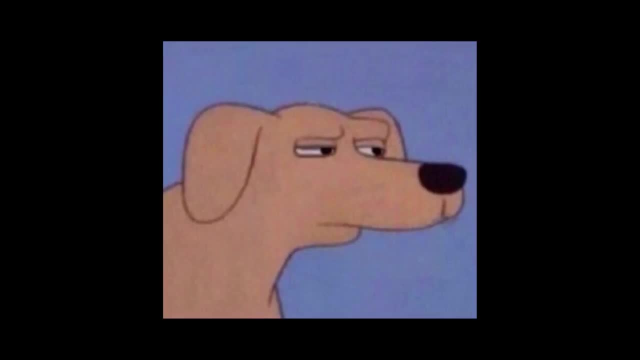 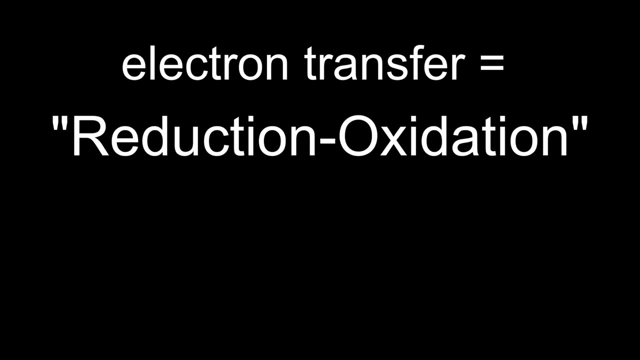 hydroxide will form water and table salt. Oh yeah, speaking of table salt, remember how it consists of ionic bonds, because sodium transfers an electron to chlorine. Well, that is called a reduction oxidation reaction or redox. If sodium chloride forms out of its pure elements, the 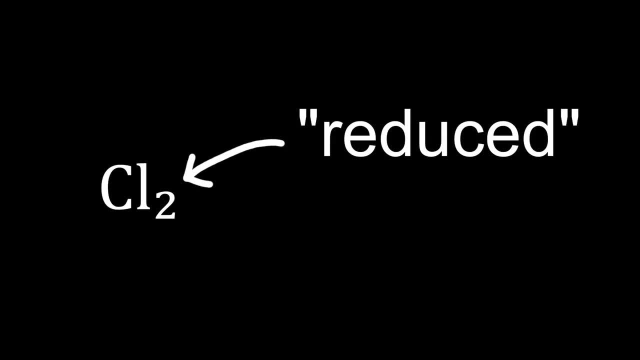 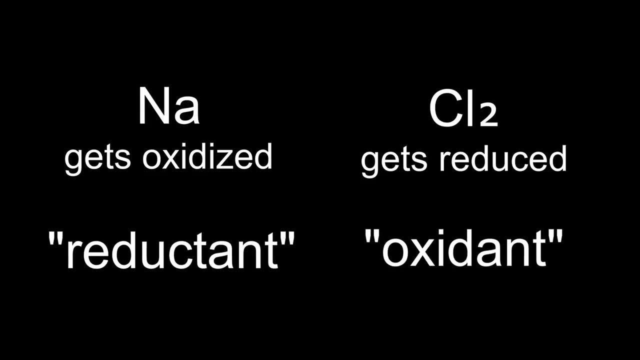 sodium gets oxidized as it loses an electron and the chlorine gets reduced as it gains an electron. Logically, sodium is the oxidant and chlorine is the reductant. Of course not, that would make sense. it's the other way around. 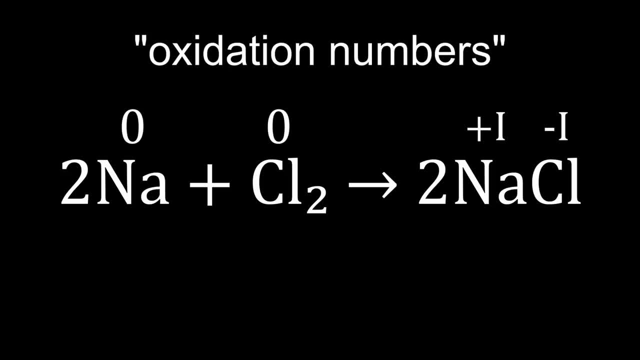 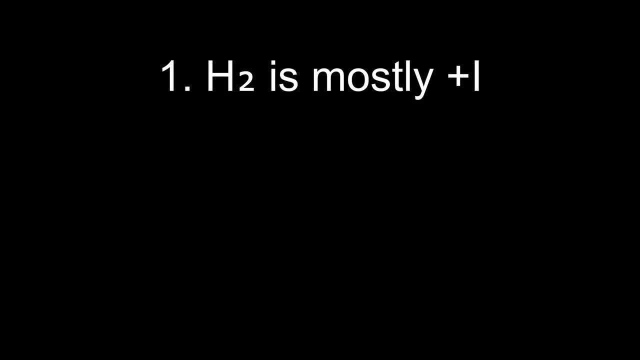 More accurately, redox reactions are reactions that change the oxidation numbers of elements, which are kind of like imaginary charges. There's just a few rules you have to know to figure those out. Hydrogen is mostly plus one. Oxygen is mostly negative two. Halogens are mostly negative one. 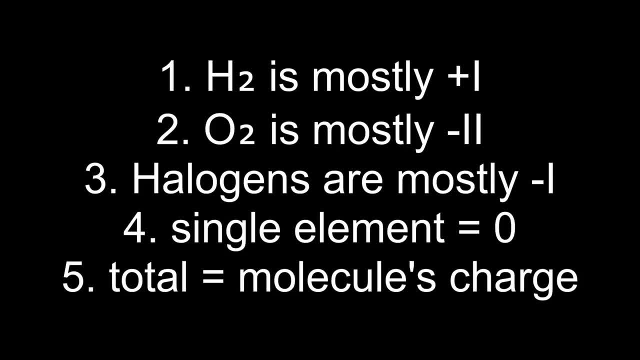 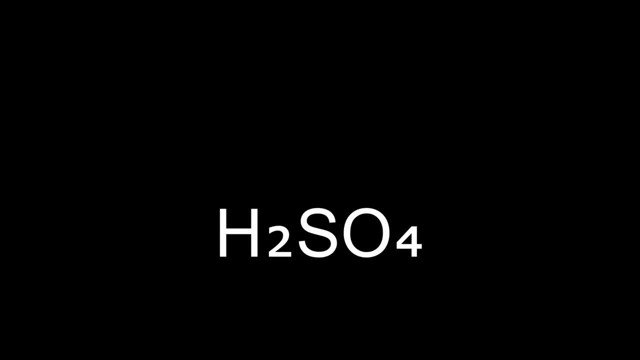 Single elements are always zero and the number of all atoms in a molecule always have to add up to the molecule's charge, So this would total zero, while single ions just have their charge as the oxidation number, For example in sulfuric acid. 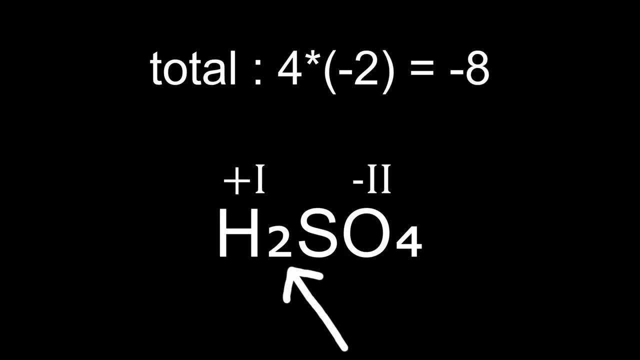 we have a charge of zero and the number of atoms in a molecule always have to add up to the oxygen. We have four oxygens, which totals negative eight. We have two hydrogens, which brings the total to negative six, and since the whole molecule is neutral, sulfur must have an oxidation number. 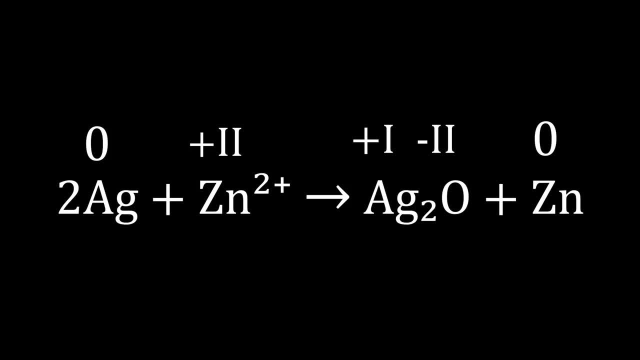 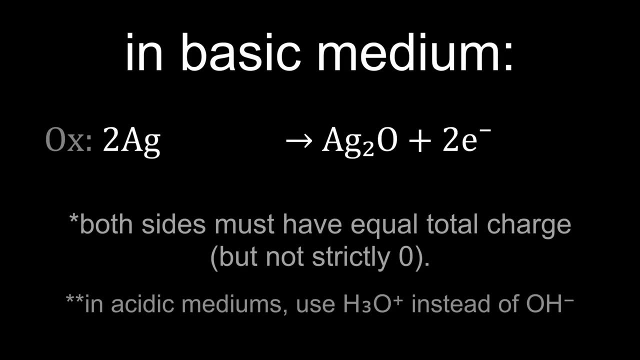 of plus six. Just by looking at the oxidation numbers of reactants and products you can deduce the flow of electrons which gives you these equations. If redox reactions happen in acidic or basic solutions, you can balance out the charges with ions and fix the stoichiometry with water. 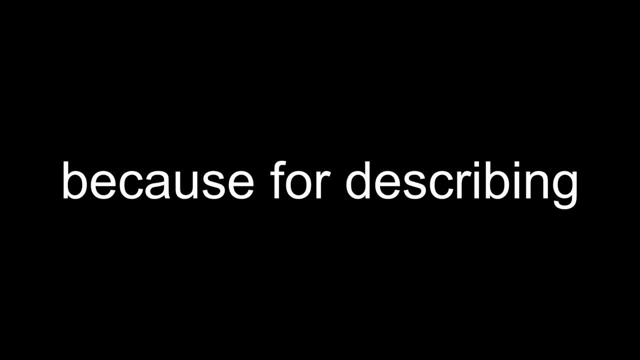 Okay, now to this weird looking thing. I spared you from it because for describing electrons, this is very simple and this is not. But this is actually like pretty wrong. Electrons don't orbit in circles. Here's how it actually works. 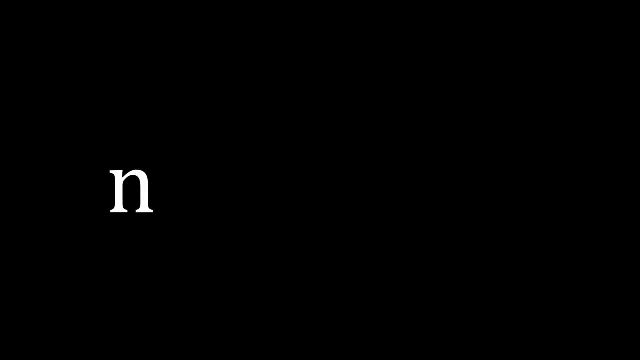 All electrons inside an atom are described by four quantum numbers: N, L, ML and MS. N corresponds to the shells, so all electrons with the same N are in the same shell. Within the shells we have subshells with multiple orbitals, which are three-dimensional regions in space where 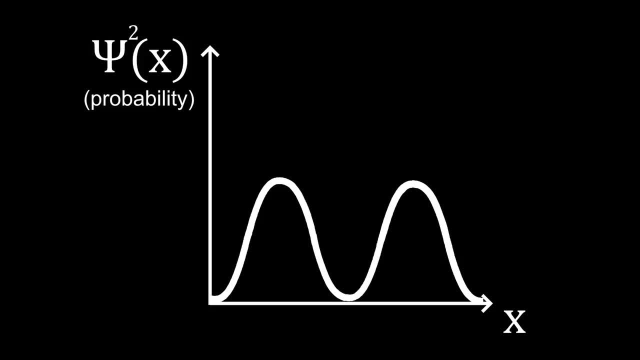 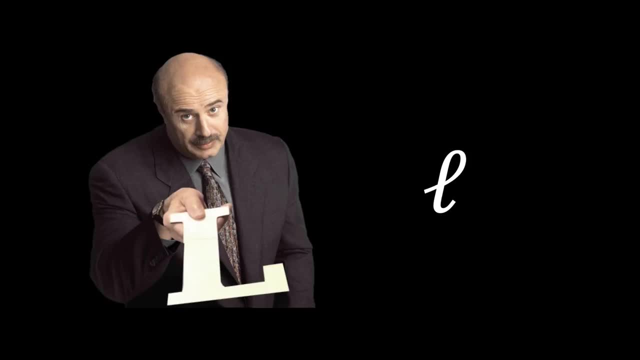 electrons could be. We know these exist thanks to Schrodinger's equation, which gives a probabilistic wave function. You can imagine it as a cloud, and the denser it is, the more likely an electron is to be there if we were to look for it. L describes the number of electrons in an atom and the 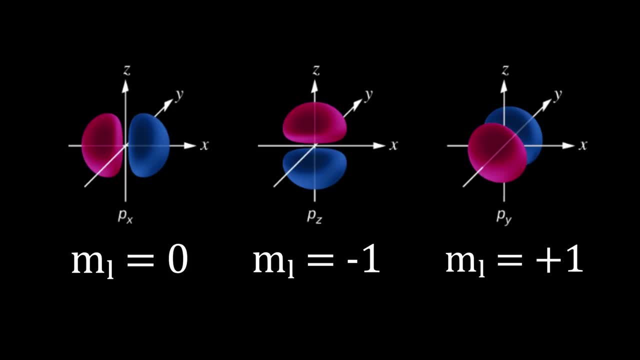 N describes the shape and ML the orientation of orbitals in a subshell. There are four subshells called S, P, D and F. If electrons have the same L, they're in the same subshell. If electrons have 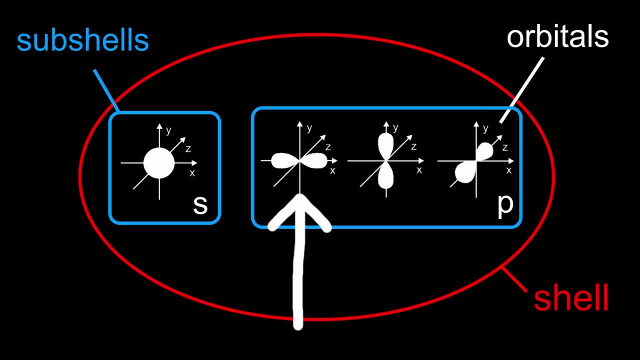 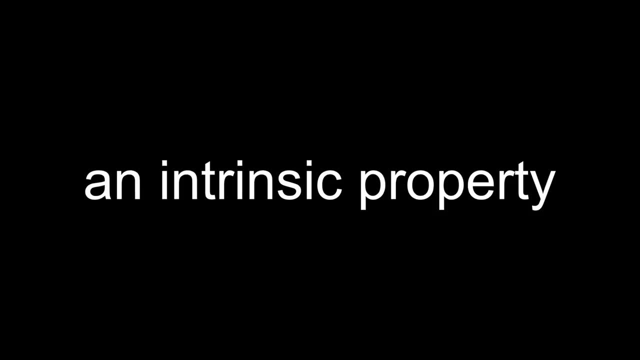 the same N, L and ML. they're in the same orbital. Also, the number of orbitals increases by two for every bigger subshell, starting at just one for S. The last quantum number describes an intrinsic property of electrons called spin, which can have two values. Some guy named Pauli said two electrons. 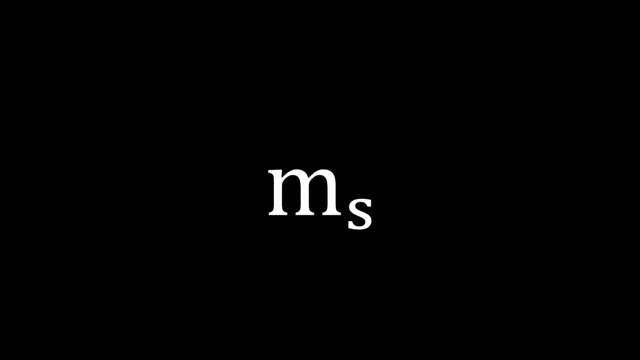 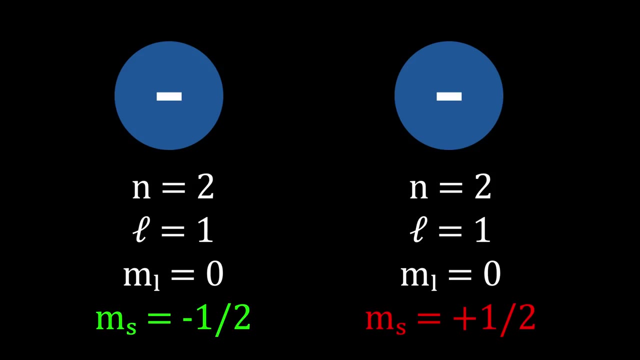 can never have the exact same quantum numbers inside one atom, Since MS can only have two values. every orbital defined by N, L and ML can hold a maximum of two electrons with opposite spin. Therefore, the S subshell can hold two electrons, the P subshell can hold six, D can hold ten.